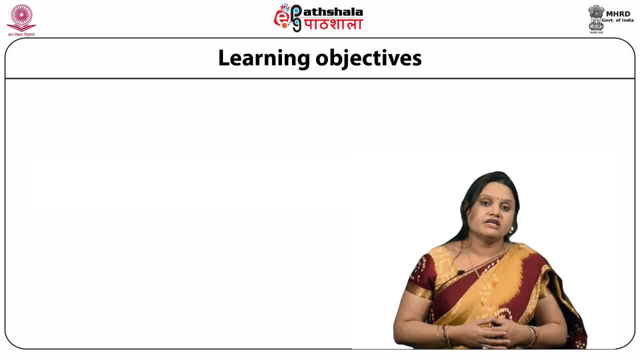 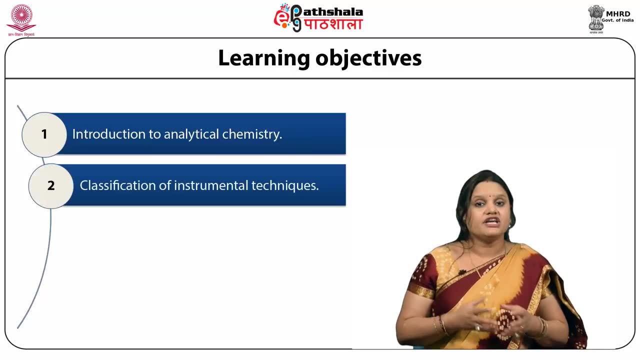 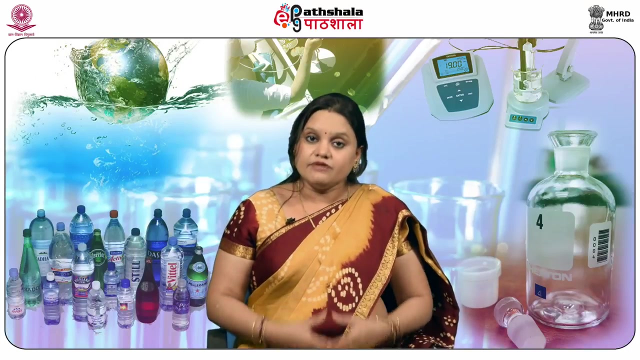 of Environmental Analysis. The learning objective of this module, including the introduction of analytical techniques, then the classification and the various types of instrumental techniques that we are using for the environmental analysis is, with special emphasis on chromatographic and the spectroscopic method, The subdivision of chemistry dealing with the quantitative 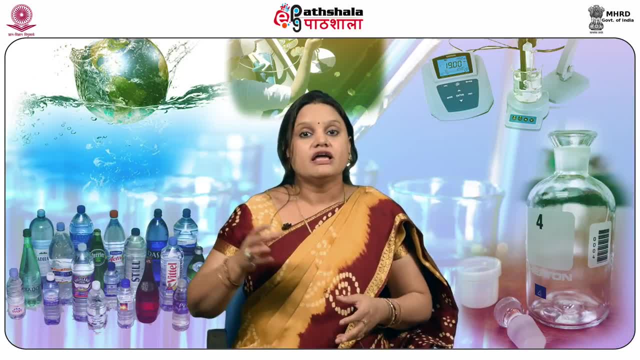 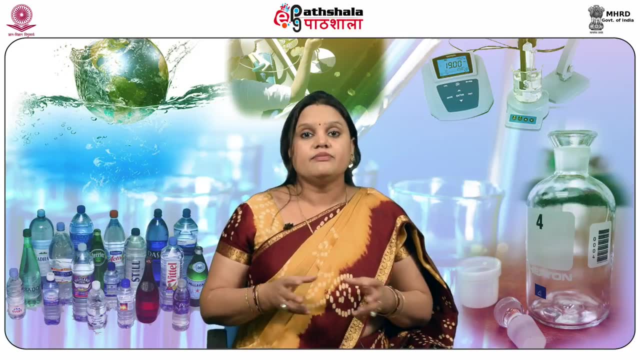 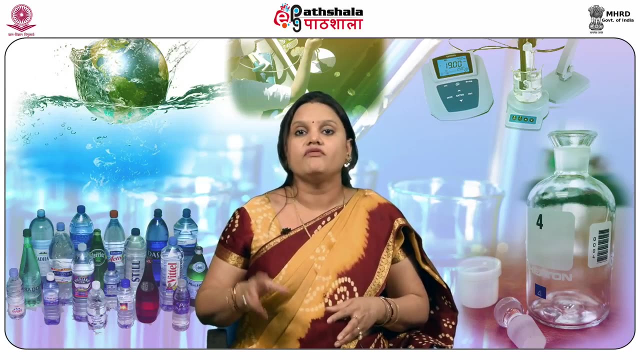 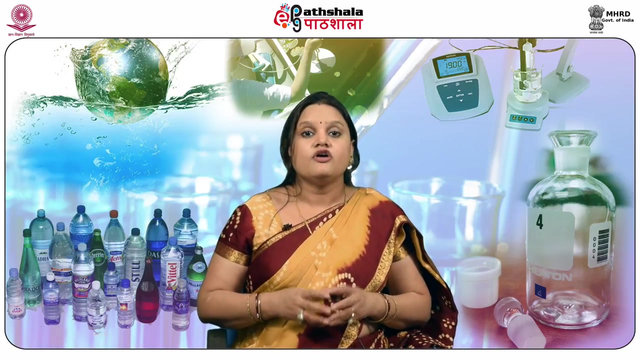 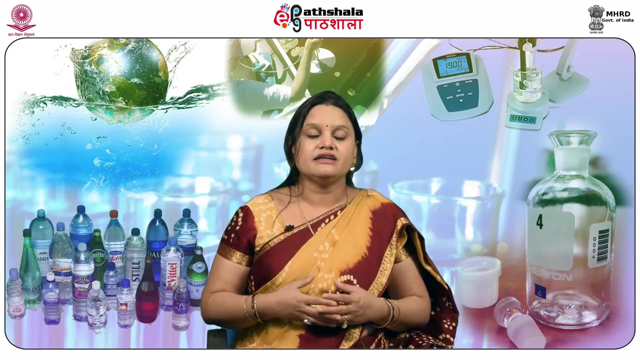 and the qualitative determination of chemical components of the substance is known as analytical chemistry. It is the branch of chemistry involved with quantitation and the qualitative identification of elements of the compounds, also called constitutional chemistry. Further, this technique is classified in two techniques, that is, number one is classical techniques. 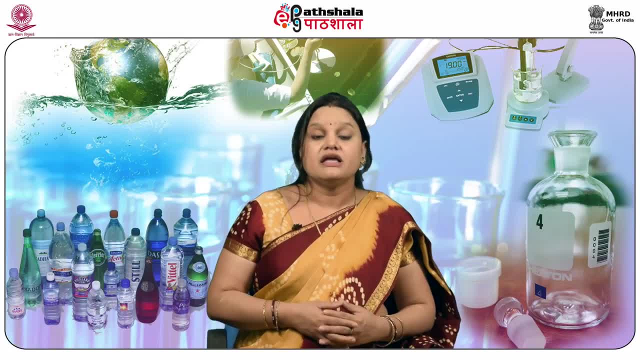 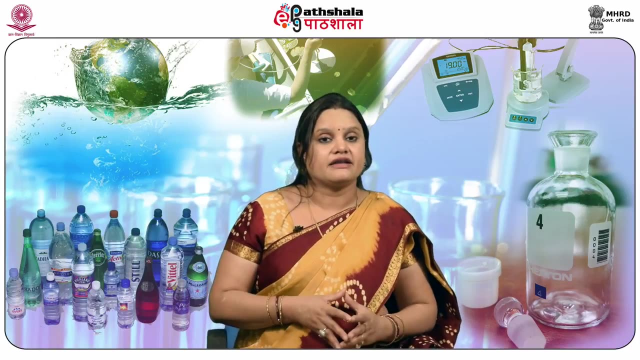 and the second one is the instrumental techniques. The acid-base indicator test, redox type of titration, is an example of the analytical chemistry carried out by the scientists. The third one is the statistical technique, which is typically defined by the second student and comes under the classical technique. Here we are going to discuss about the various 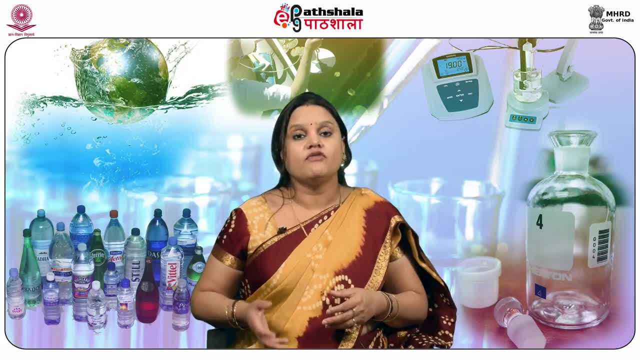 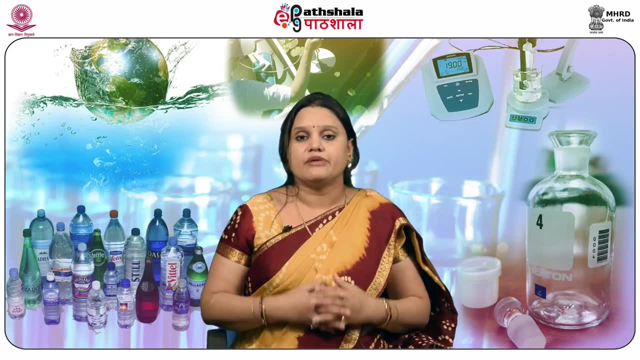 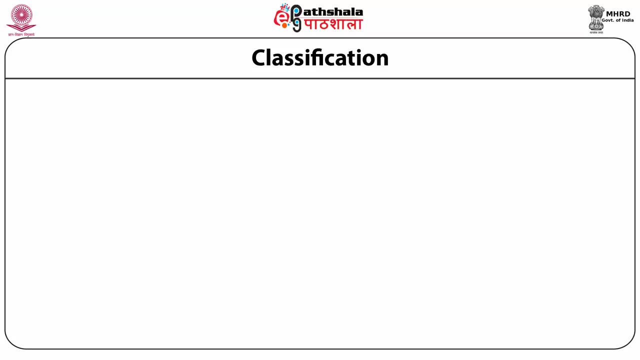 instrumental techniques used for the analysis of environmental pollutants present in the either in the air, water or soil sample. Now we discuss here about the classification of analytical chemistry. The analytical chemistry is classified about their application by the chemical class which is known as an analytical chemistry. The analytical chemistry is classified. 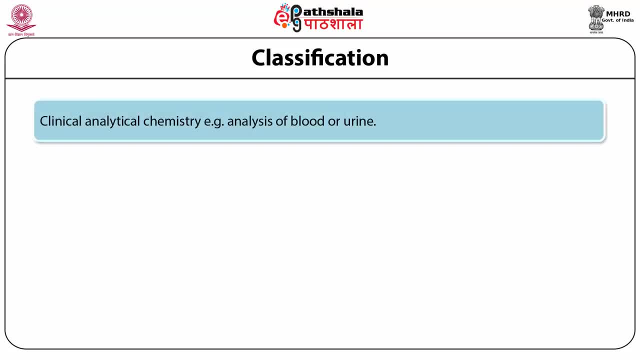 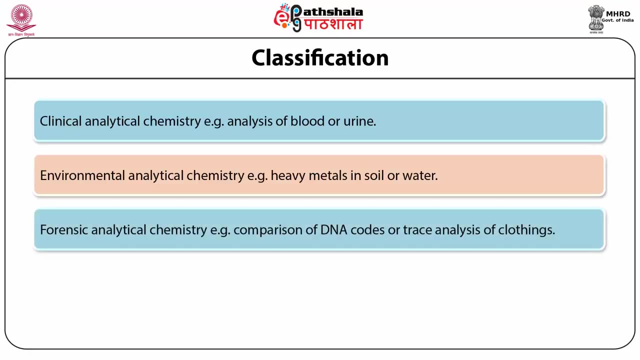 about their application, and this classification of analytical chemistry is known as an analytical part in clinical analytical chemistry, for example, the analysis of blood or urine. then the environmental analytical chemistry, for example analysis of heavy metals or the pesticides in soils and water. then the forensic analytical chemistry, including the comparison of dna codes. 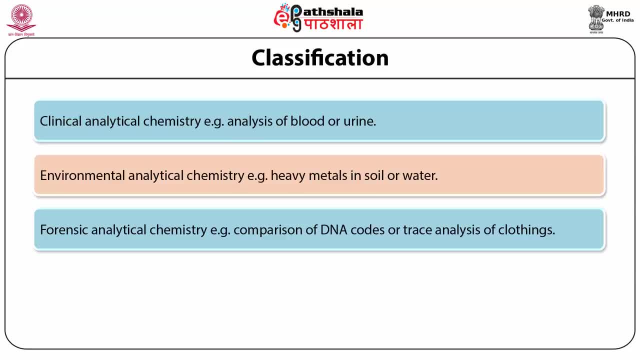 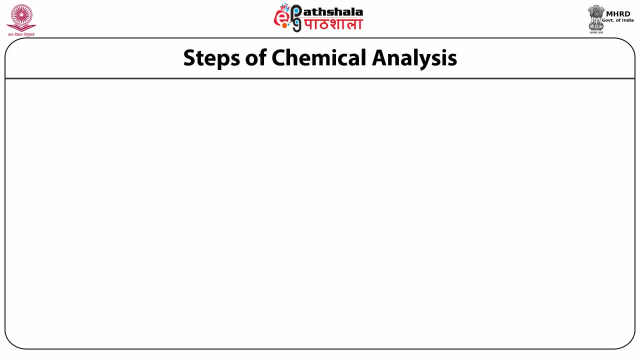 or trace analysis of clothing, and it is also used in the quality control process, for example, the analysis of vitamin contains in food sample. the steps of chemical analysis, including sampling, sample naming, sample preparation analysis, signal recording, signal processing, then the family analysis, the birthmark analysis, the chemical analysis for the content analysis. 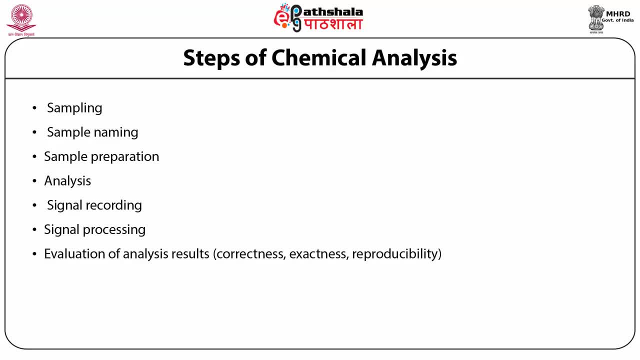 we had in this process can always be ecosystem analysis, then sample operation analysis, such that then the final analysis after the final period and that's the beginner analysis. now you can evaluation of analysis result like correctness, exactness and the reproducibility, then plausibility. 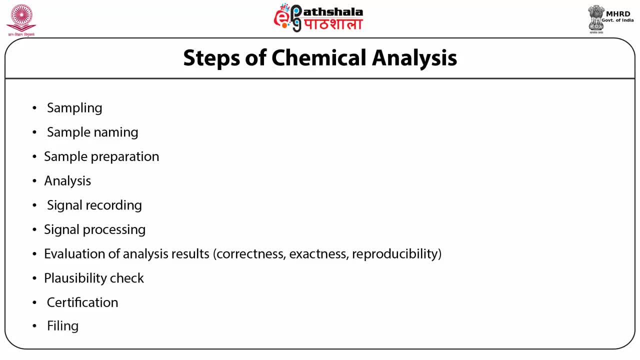 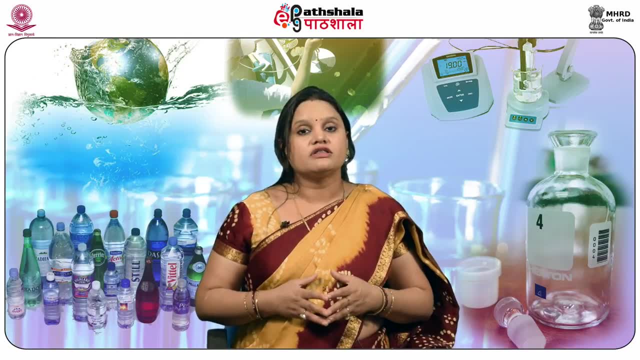 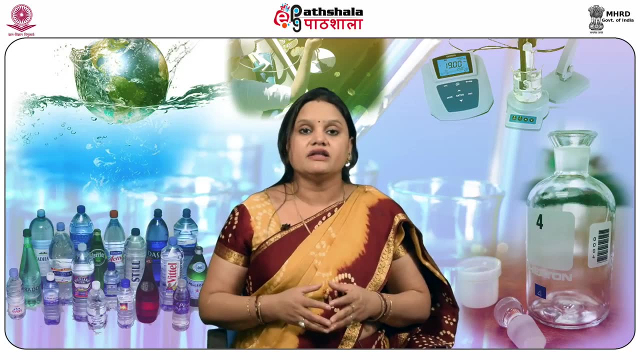 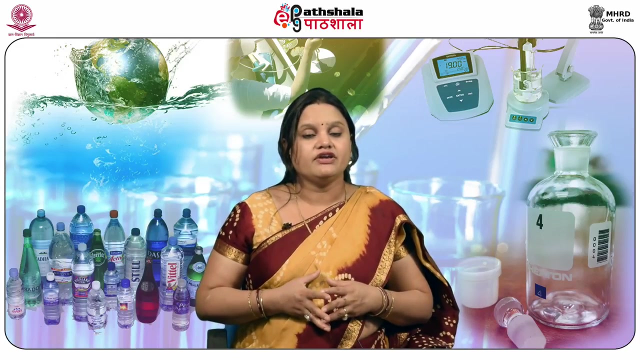 check, certification and filing. Here we are discussing about the various instrumental technique used for the environmental contaminant analysis. There are many instrumental techniques which are applied in the environmental analysis, including chromatography, various types of chromatography. that includes gas chromatography, high performance liquid chromatography like 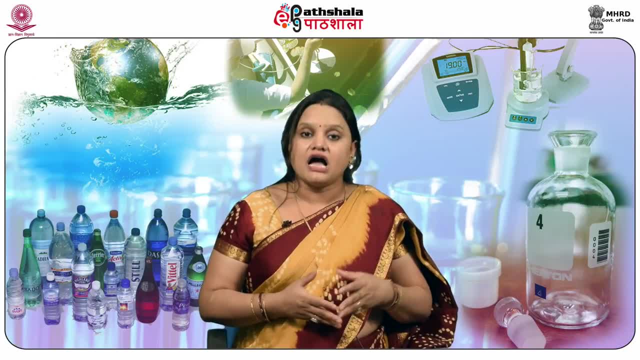 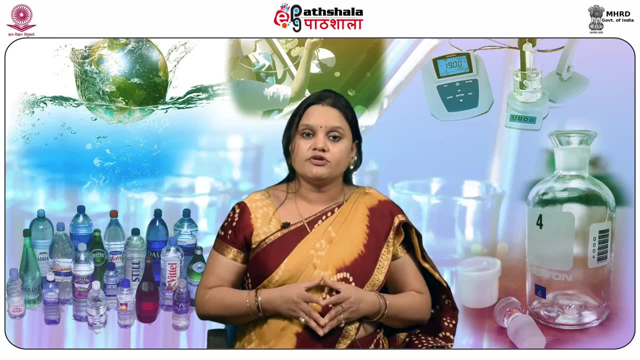 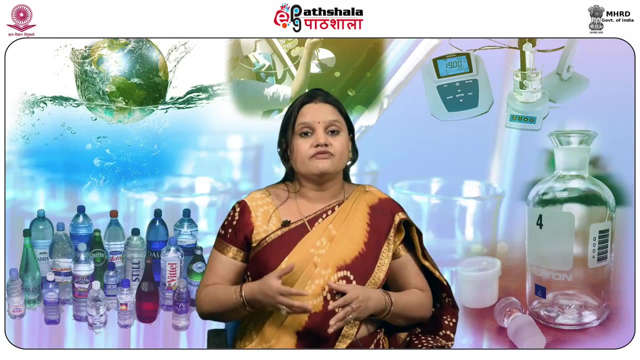 that is, HPLC ion chromatography, thin layer chromatography, supercritical fluid chromatography, size exclusion chromatography and capillary electrophoresis and electrochromatography- The other methods which are most frequently used for the environmental sample analysis. is the spectroscopic techniques that, including the UV, visible absorption spectroscopy, infrared spectroscopy, fluorimetry and chameleuminescence, X-ray fluorescence, spectrometric method, atomic absorption and the flame emission spectroscopic method, atomic emission, spectroscopy and the. 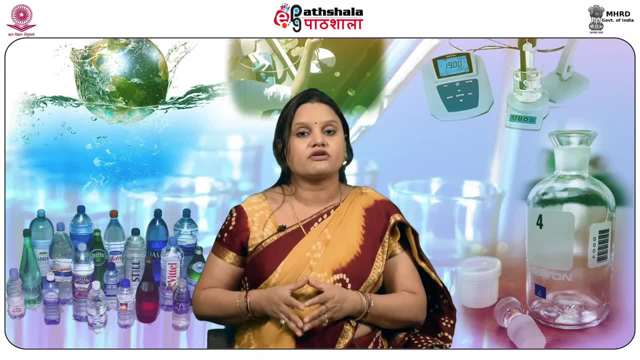 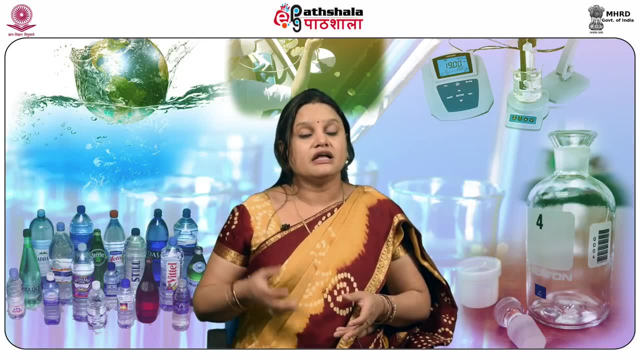 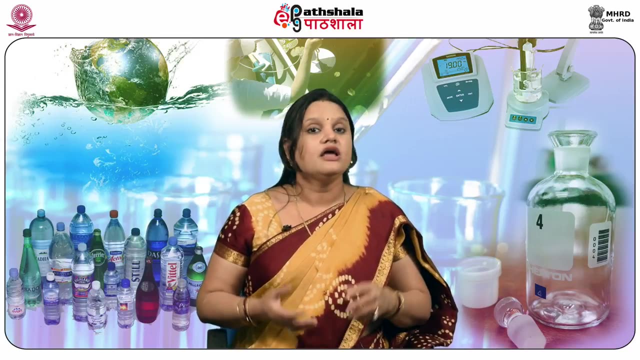 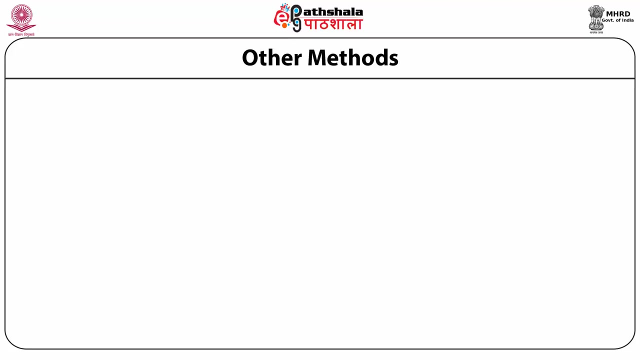 nuclear magnetic resonance spectroscopy, that is NMR. Apart from these two major techniques, the other methods that are used nowadays for the contaminant analysis, including mass spectrometry, potentiometric method and voltammetric and coulometric method. Now we discuss here about the chromatographic techniques. The chromatography is the process. 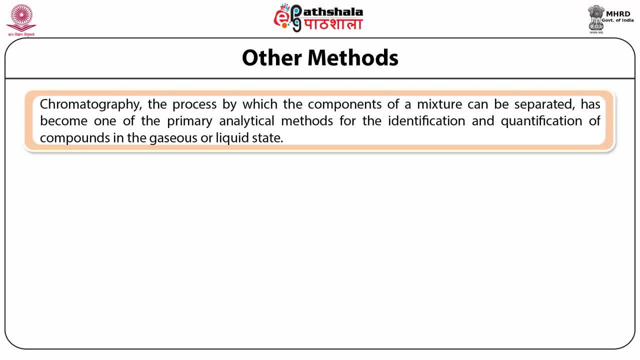 by which the chromatography is performed. The chromatography is the process by which the chromatography is performed. The chromatography is the process by which the chromatography is performed. It is the process that supports the chromatography and causes the result. The chromatography types are generally occurred according to thestromatic scale��icム. 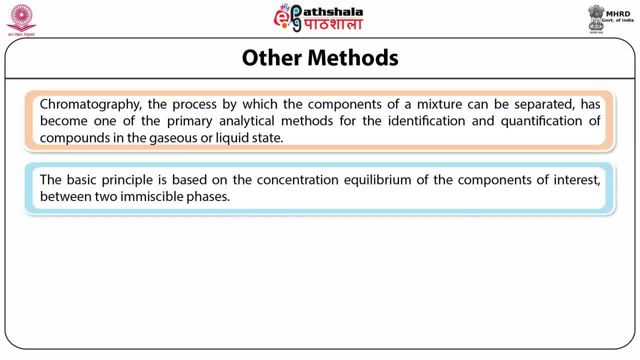 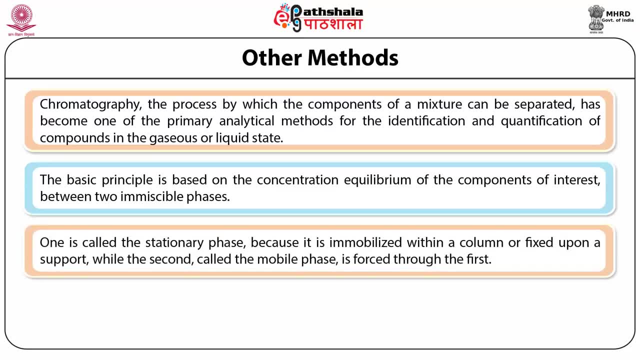 and HV. It is the process by which cur, but it can also Levatoreten murderer factor: stationary phase, because it is immobilized within a column or fixed upon a support, while the second one is known as a mobile phase, that is forced through the first. the phases are chosen such that 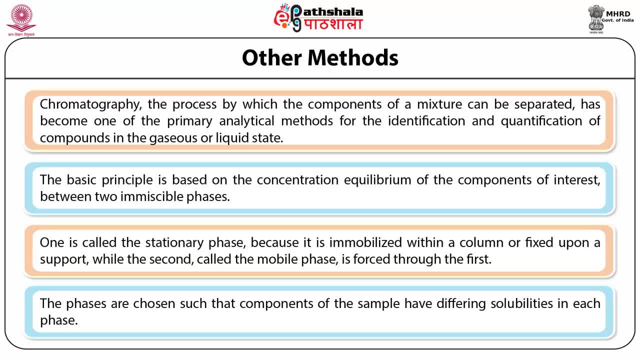 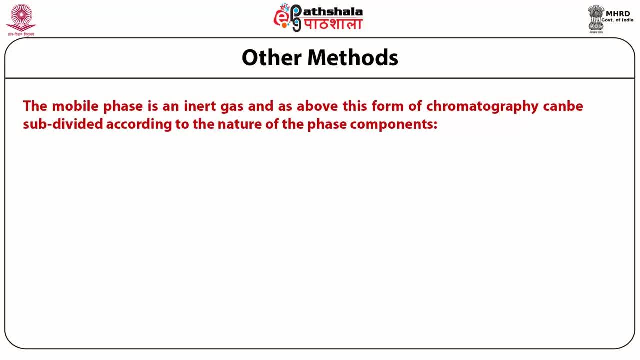 components of the sample have differing solubilities in each phase. the mobile phase is an inert gas and, as above, this form of chromatography can be subdivided according to the nature of the phase components. the number one of the chromatography technique is known as the gas or the liquid chromatographic technique, that is, glc- gas liquid. 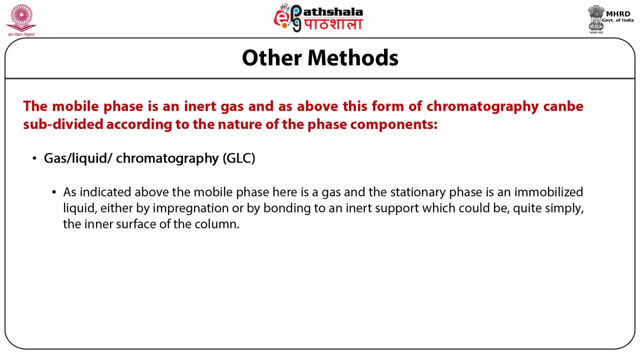 chromatographic technique. as indicated above, the mobile phase here is a gas and the stationary phase is an immobilized liquid, either by impregnated or by bonding to an inert support, which could be quite simple, and inner surface of the column. this is the technique that commonly called gas phase chromatography, that is, GC. the second. 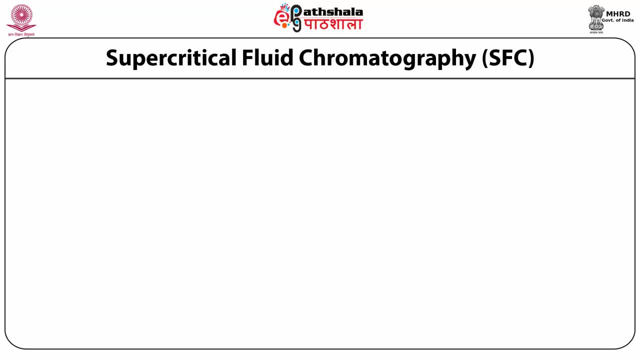 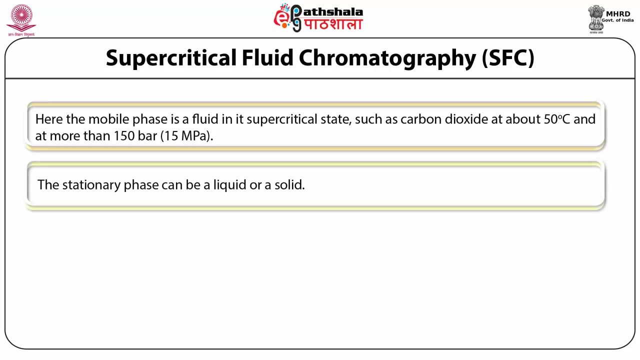 chromatographic technique that is used in for the analysis of environmental sample is the supercritical fluid chromatography. here the mobile phase is a fluid. in it supercritical state, such as carbon dioxide at about 50 degree centigrade and it more than 150 bar. the stationary phase can be a liquid or a. 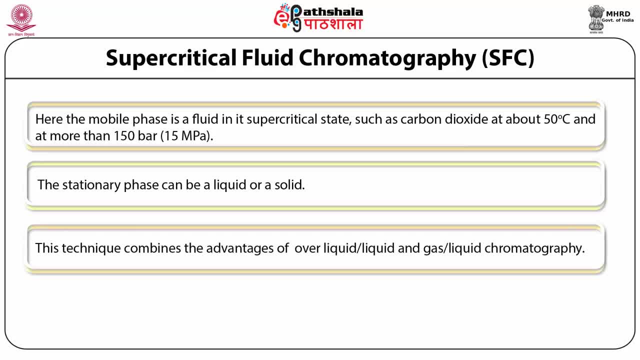 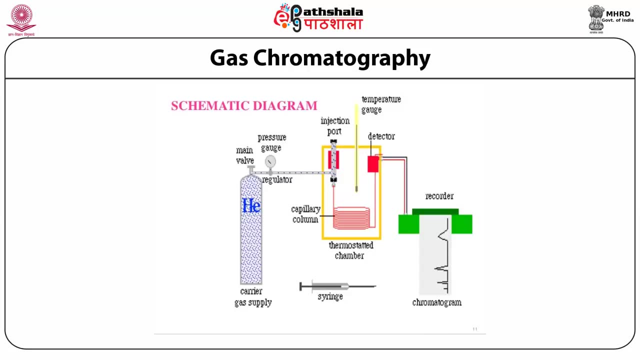 solid and this technique combines the advantages of over liquid liquid and gas liquid chromatography. here this finger shows the school metallic presentation of a gas chromatography. there is a carrier gas supply, that inert gas that is the mobile phase throughout the system. generally nitrogen, helium organ are used as if carrier gas in the gas DC, but the most 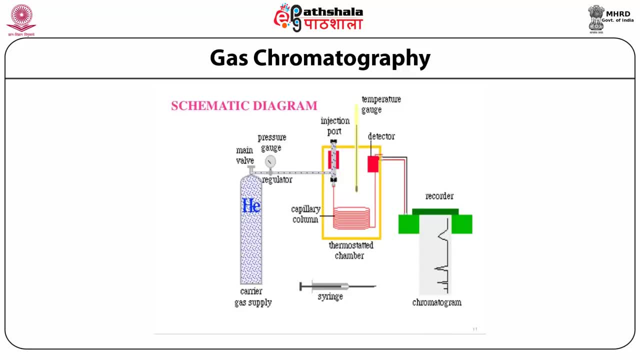 frequently used or most versatile use: inert gases, nitrogen for the gas chromatography chromatograph. This flow rate of the gas is maintained by the pressure goes or the regulator, and then it is transferred to the column and then it goes to the detector and then the recorder. 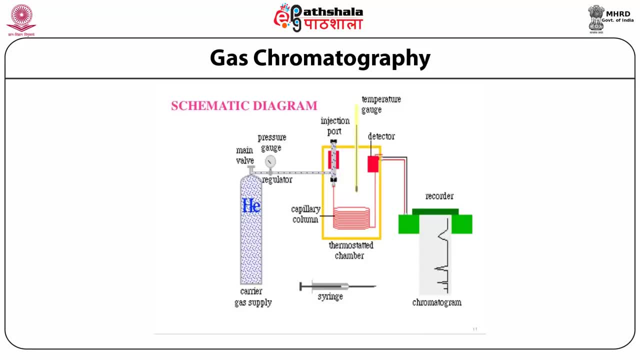 recorded the flow of the mobile phase as well as the sample present in the mixture In the injection port. when the system is totally saturated with the nitrogen, then the sample is injected into the column and the temperature of the injection port oven and the detector cap enough high so that 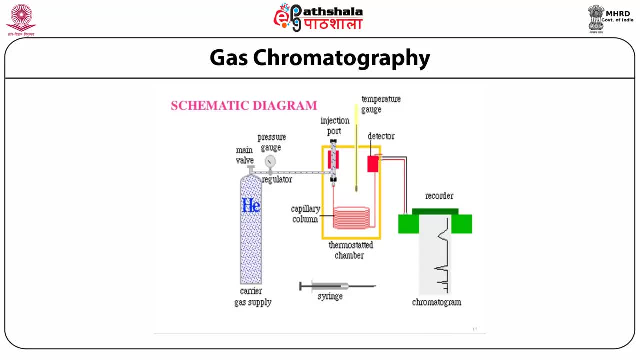 all the ions components that are present in the solution is ionized properly, and these ionic forms or the gases are then transported to the column that is housed in a oven and where the separation of these ions takes place. then they are finally detected by the detector. 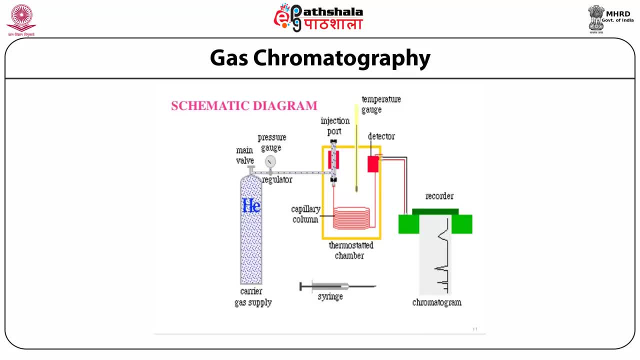 Here you can see that the ionic form is being transferred to the detector and then the sample. here are various type of specific detectors used in the GC for the recording the various types of pollutants in the environment, For example, like electron capture detector is used for the 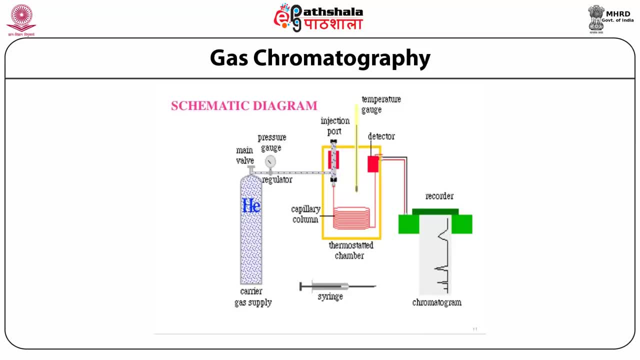 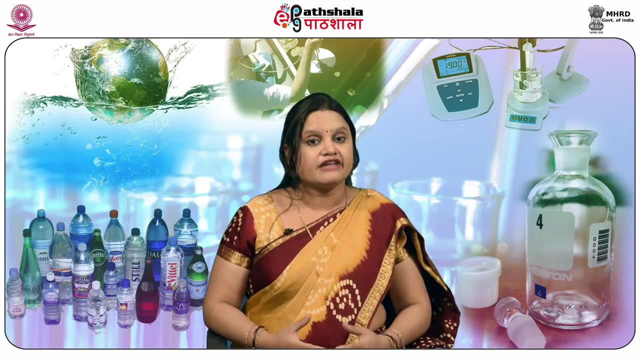 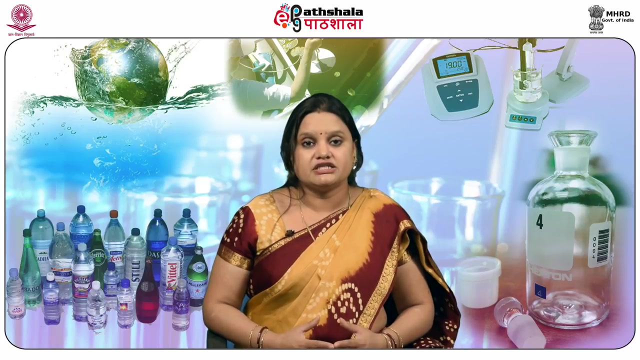 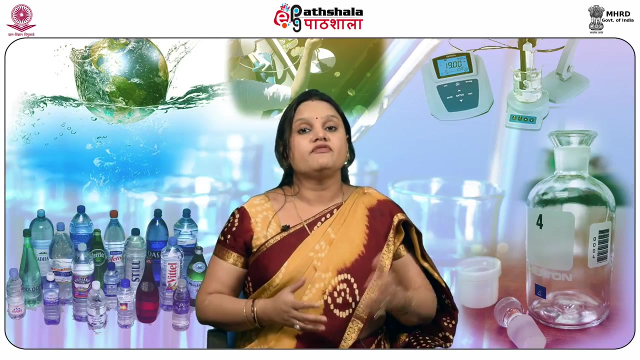 determination of pesticide and the flame ionization detectors are used for the determination of hydrocarbons present in the air. Now we are going to discuss here the second most important methods of environmental contaminant analysis, that is, high performance liquid chromatography, also known as HPLC. Of all the chromatographic techniques whose mobile phase is a liquid, high performance liquid. 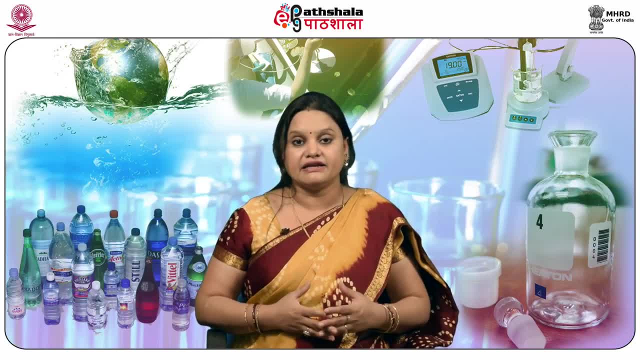 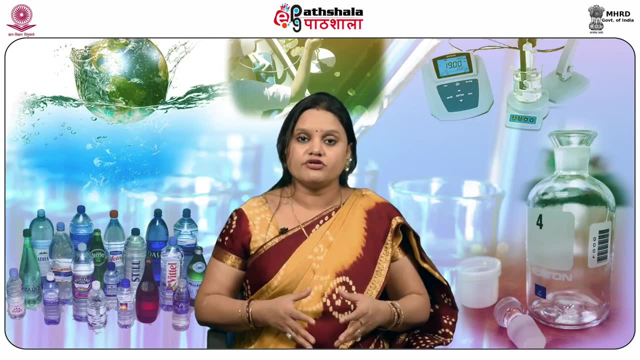 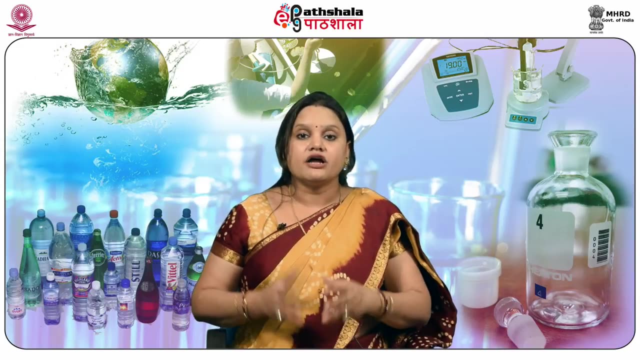 chromatography is perhaps the best known technique. Its fields of application overlaps a large section of gas phase chromatography, to which can be added the application of the gas phase chromatography. It can detect the analyte of many compounds that are thermolabile or very polar or of a high molecular. 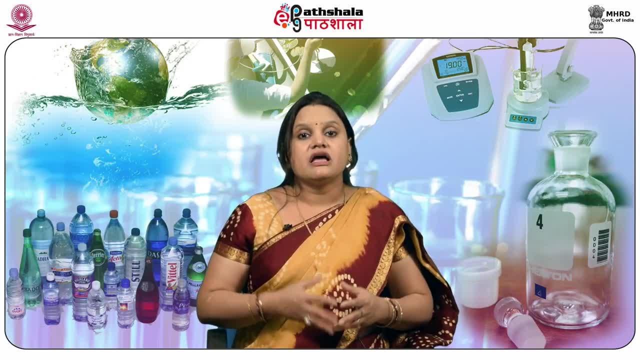 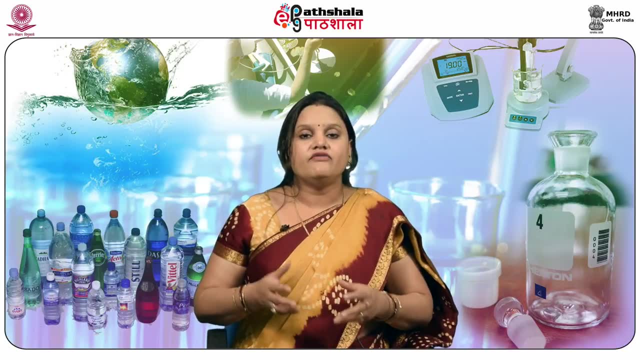 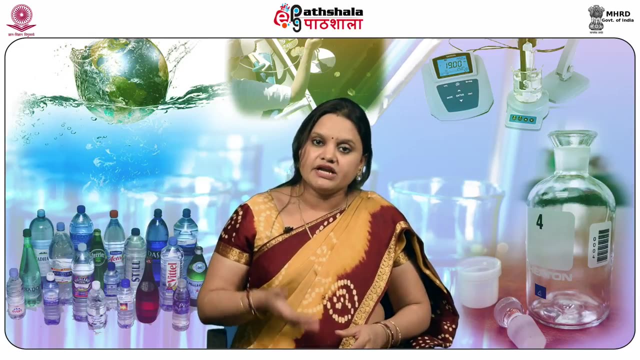 weight substances, Its sources, is also due to the possibility for the chromatographer to act in a very precise manner upon the selectivity between the compounds through an appropriate choice of columns and eluent compounds. In addition, the chromatography of the chromatography of the liquid chromatography- 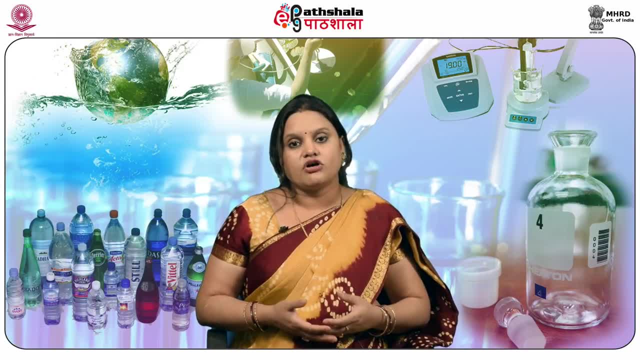 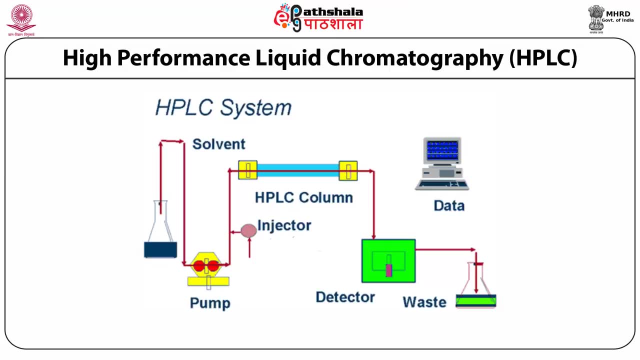 composition by exploiting the solute mobile phase or the stationary phase interaction. Here is the schematic representation of the high performance liquid chromatographic system, where the mobile phase is liquid, so it is tapped in a solvent container, from where the solvent is passed through the column by using the pump. then pump maintain the constant flow. 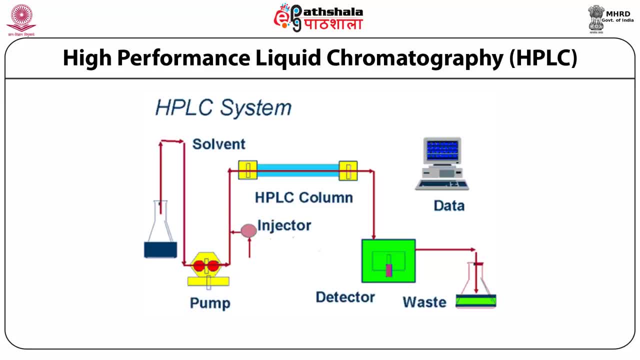 rate of the mobile phase throughout the column. here the column are used are small in size as comparative to GC, and when we inject the sample then this carrier, mobile liquid mobile phase, carry out the sample throughout the HPLC column where the separation of the species takes place, and after that the detector gives the shows the sensitivity of that particular. 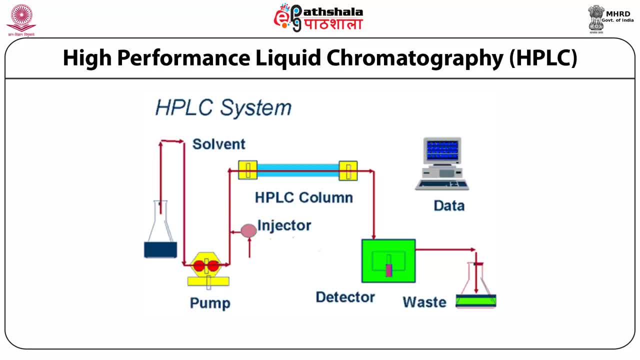 compounds and detect the sample, The signal of the contaminants that are present in the sample. and the major advantage of this technique is that the waste is collected by after the determination of this method, so that we can collect here an important products or byproducts from the environmental sample. 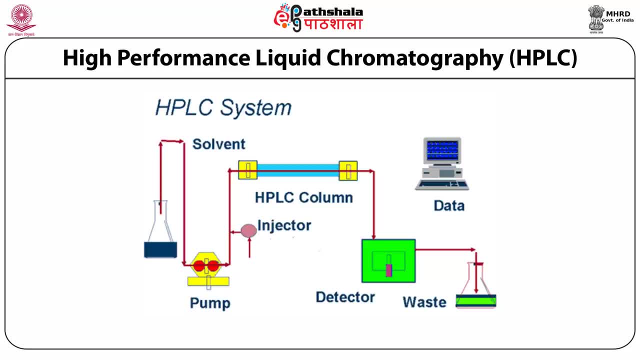 The best example of the determination of environmental contaminants through the HPLC that, including the various types of pharmaceuticals That are present in the environment, then the other contaminants, like various other, like advanced pesticides, like organophosphate carbamates, can also be detected by using HPLC techniques. 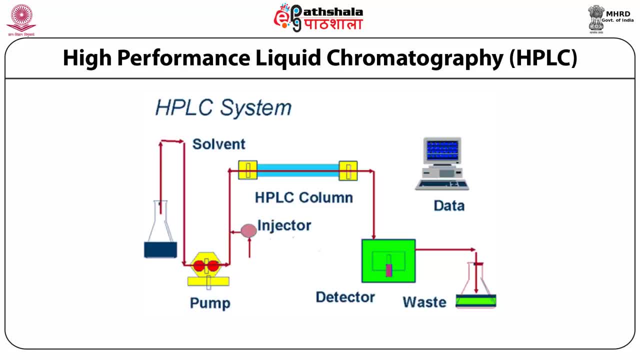 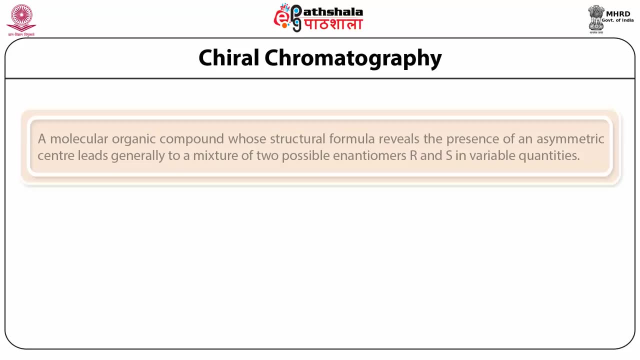 and many more compounds which are thermally unstable that can be analyzed by using HPLC technique. The third one important thing is that when we use the HPLC technique, we can also detect the presence of these chemicals. The third one is that the chromatography of the chromatography is known as chiral chromatography. 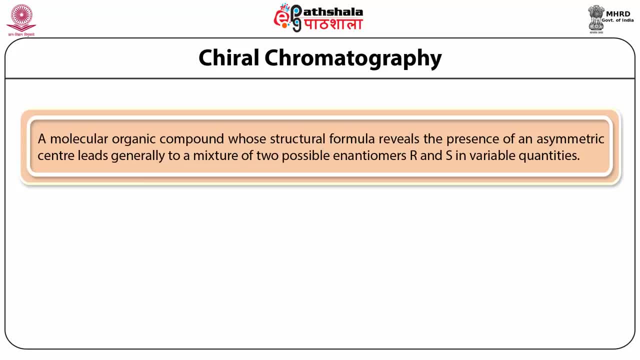 A molecular organic compound whose structure formula reveals the presence of an asymmetric center leads generally to a mixture of two possible enantiomers, that is, R and S, in variable quantities. If such a mixture is chromatographed on a column packed with a chiral stationary phase, 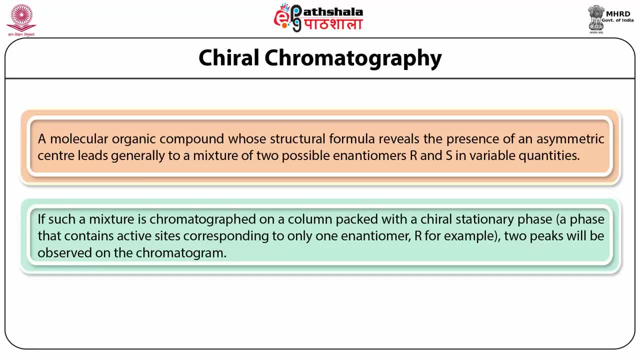 Then the chromatography can be analyzed. The chromatography of the chromatography is known as chiral chromatography. The chromatography of the chromatography is known as chiral chromatography. phase A- phase that contains active sites corresponding to only one enantiomer are for: 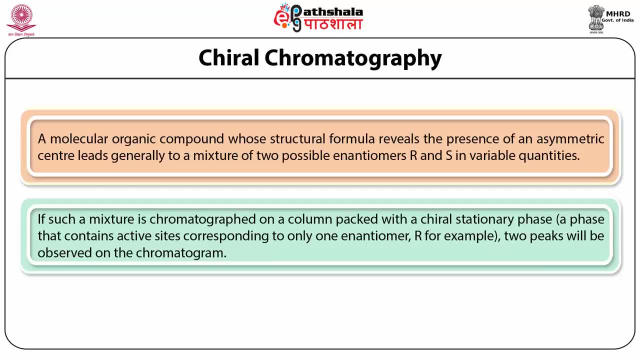 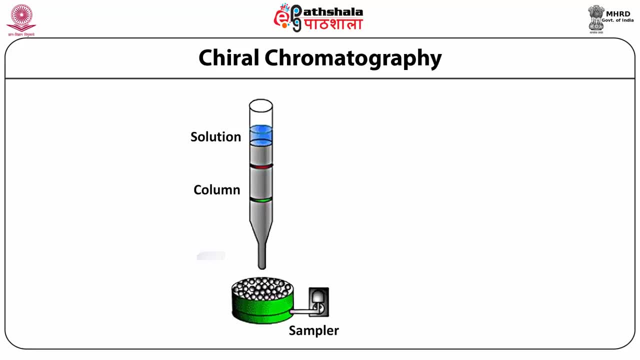 example, and the two peaks will be observed on a chromatograph. Here is the picture of separation through the chiral chromatography of the compound When the solution pass through the column. the column is made up of silica gel and here the chiral compounds are separated. 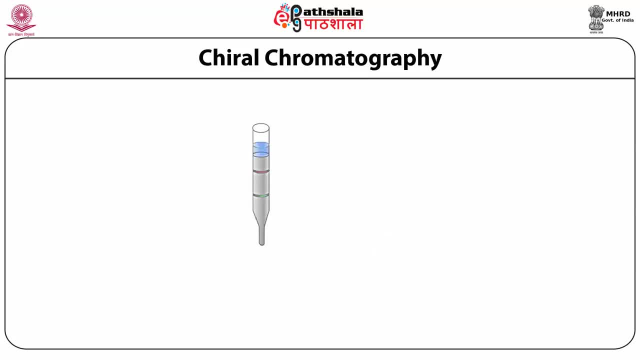 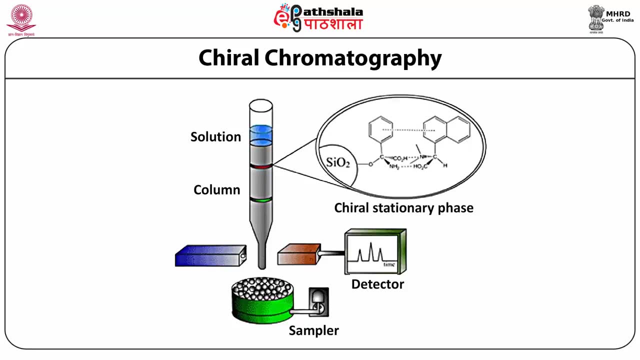 out by using the specific type of mobile phase, and then these chiral compounds are collected, pass through the detector column and then detected by the detector. The sample of the compound is also collected and it can be recovered by the passing solution. The example of the 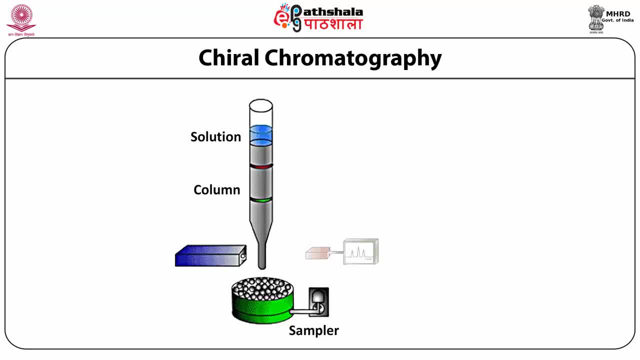 such kind of determination is the enantiomer of some glucose containing compounds and the determination of these compounds in a blood sugar level or their determination in the plasma. also, that we can done by using this chiral chromatography. The next one is the ion chromatography. The ion chromatography is a separation technique. 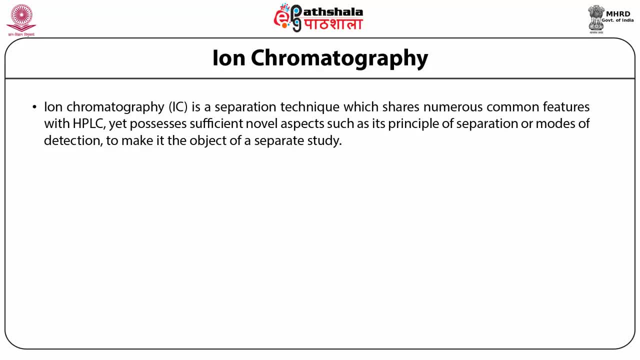 which shares numerous common features with HPLC, yet possesses sufficient nobel aspects, such as diğer principal of separation or modes of detection, to make the object of a separate study. Ion chromatography is adapted to the separation of ions and polar compounds. The mobile phase, composed of an active substrate shaped like 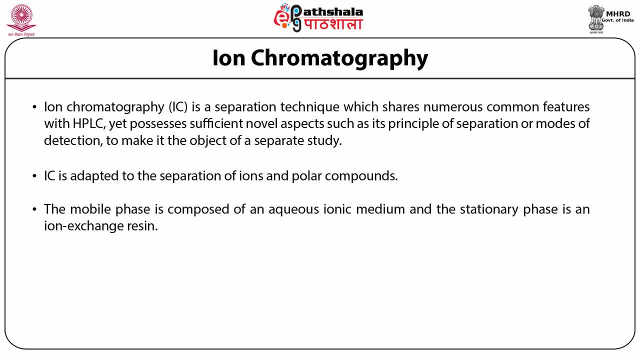 an map vibrates at an line. Ion chromatography is adapted to a separation of ions and polar compounds. The mobile phase is composed of an active ĩ aqueous ionic medium and the stationary phase is an ion-exchange resin. Besides the detection methods based on the absorbance or the fluorescence, ion chromatography 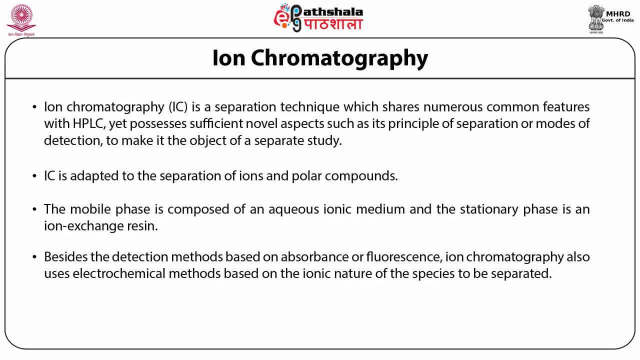 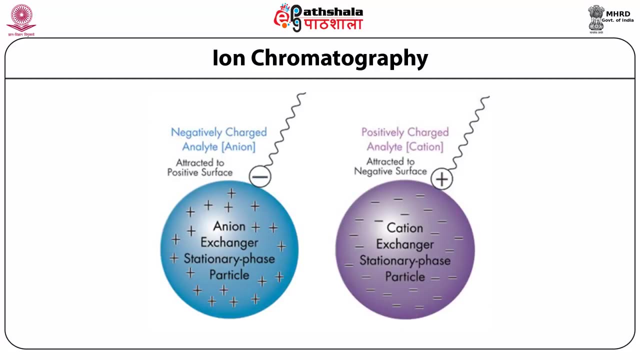 also uses electrochemical methods based on the ionic nature of the species to be separated. Its greatest utility is for the analysis of anions for which there are no other rapid analytical methods. Here in this picture, the anion exchanger stationary phase particle and the cation exchanger stationary 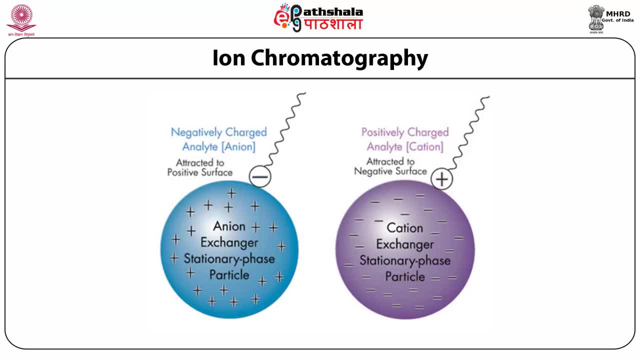 phase particles are observed Where, if it is anion exchanger stationary phase particle, they attracted the positive or negative ion from the solution And the metals, the anions like chloride, sulphide and the other ions that are present in the water attached to this stationary phase, and then you can identify the presence of. 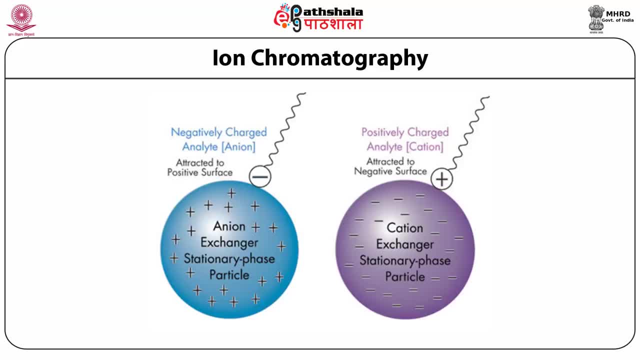 anion by using the anion presence of cations, by using this anion exchange stationary phase. Similarly, the various metal ions are also determined by using the cation exchange stationary phase particle and we can classify or detect the trace amount of heavy metal present in. 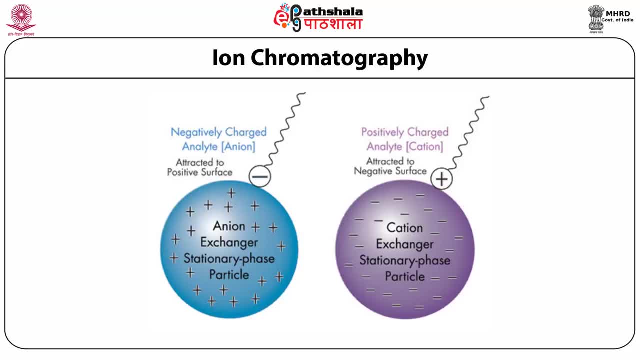 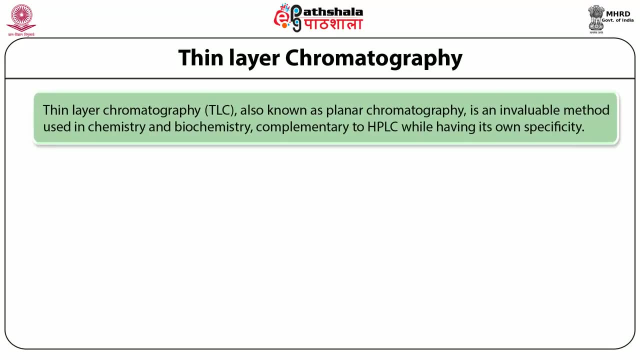 the water by using ion chromatography. The next one is the thin layer chromatography. The thin layer chromatography, also known as the planar chromatography, is an invaluable method used in chemistry and biochemistry, complementary to actual chromatography. It is used in the construction of HPLC, while having its own specificity. 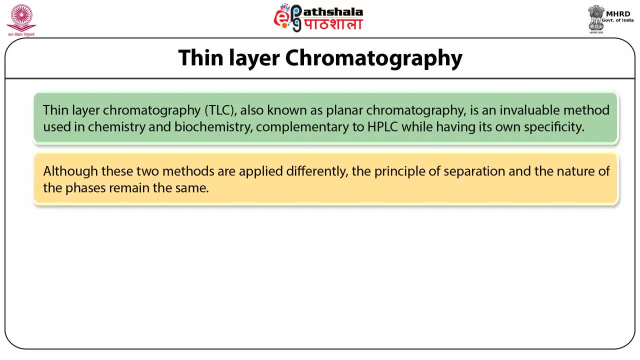 Although these two methods are applied differently, the principle of separation and the nature of the phases remain the same: Cheap and sensitive. this technique that is simple to use can be automated by using the advanced thin layer chromatography. It has become essential, principally since it is possible to undertake specific studies. 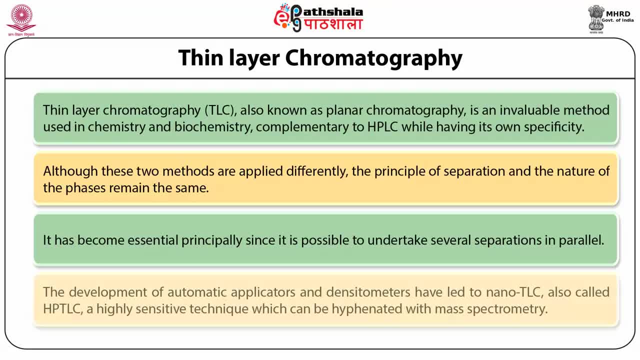 on this. several separations in parallel, the development of automatic applicator and the densitometers have led to the nano tlc and also known as hptlc, that is, high performance thin layer chromatography. it is a highly sensitive technique which can be hyphenated with mass spectrometry. 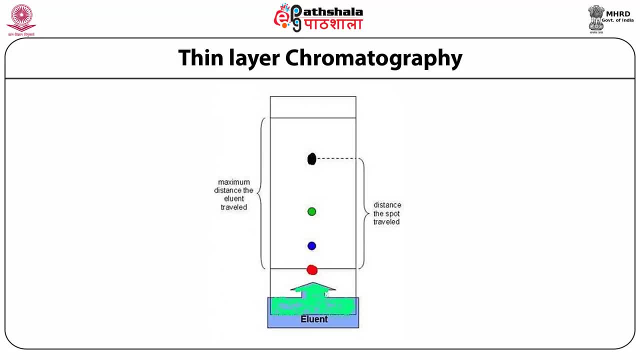 this is the picture of the thin layer plate from where, when we spotted a sample and then dip into the element, then the element is passes through this plate due to the capillary action or by the force of gravity, or the distance traveled by the spot is calculated and this 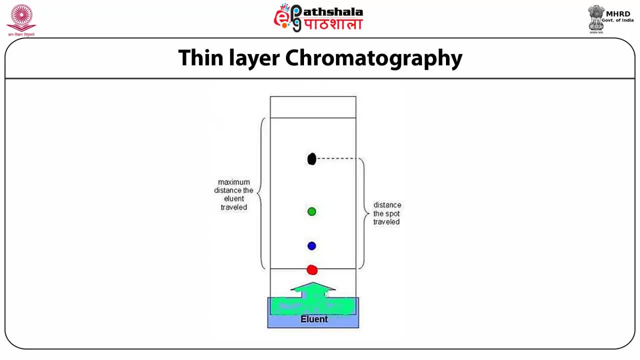 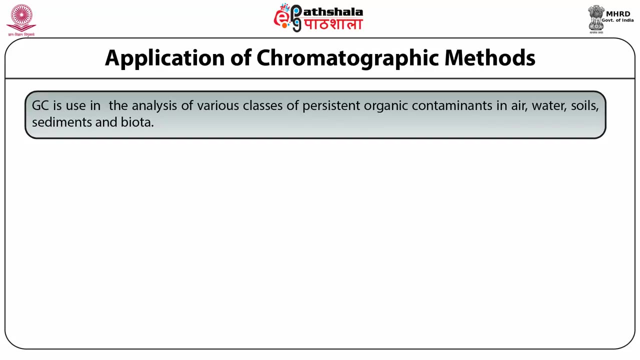 is the qualitative parameter of any species present in a solution. now we discuss here about the applications of chromatographic method. GC is used in the analysis of various classes of persistent organic contaminants in air, water, soil, sediments and the biota. the organic pollutants groups covered are volatile organic compounds, polycyclic aromatic hydrocarbons. 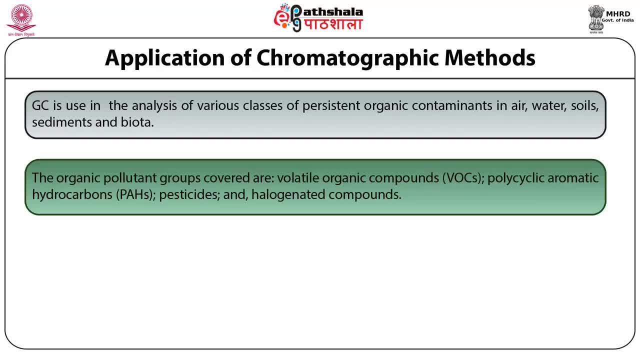 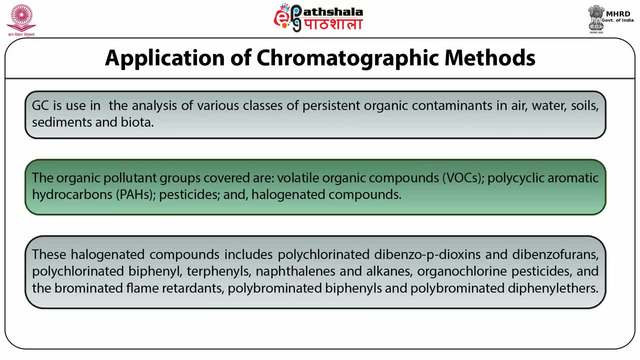 pesticides and halogenated compounds. these halogenated compounds includes polychlorinated dibenzoparadioxin and dibenzofuranes, polychlorinated biphenyls, terpenyls, naphthalenes and alkynes, organochlorine, pesticides and the brominaited flame retardant, polybrominated biphenyls and. 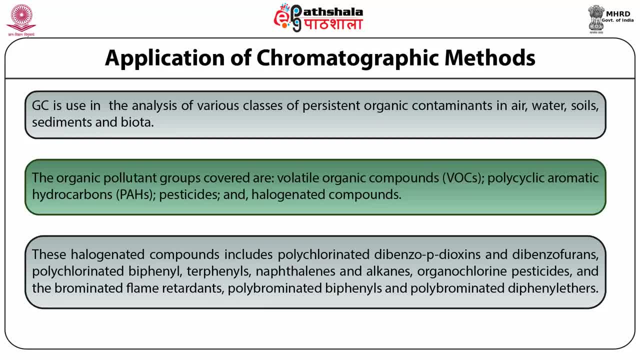 polybrominated diphenyl enters as a contaminant in a water and air water solution, both combinatoruz gates by fl, deploy walls and sewersung the air part from this. the other techniques of like HPLC chiral chromatography are also used. 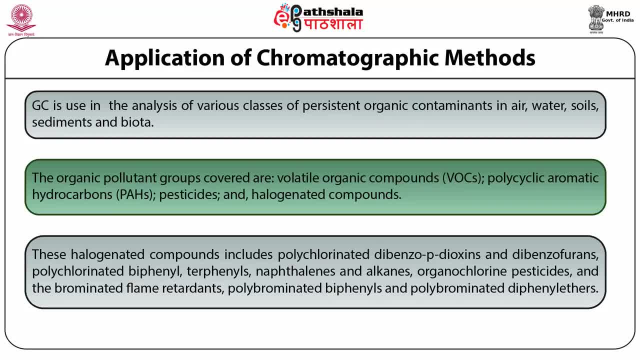 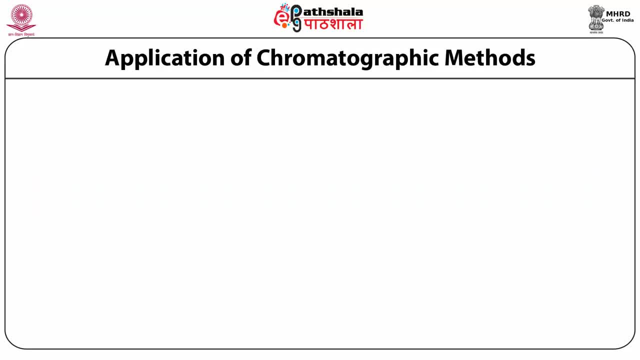 for the analysis of pharmaceutical and some pesticides and fertilizers in the soil and the water sample. the next application of the chromatographic techniques, including the fingerprinting oil spills. one of the more demanding applications for chromatography is the fingerprinting of oil products associated with oil spills at sea. 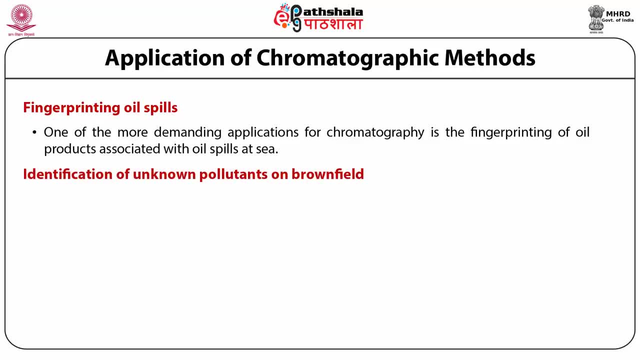 then the identification of unknown pollutants on brown field. the brown field sites can also contain unknown polymeric materials which require identification so that they can be disposed of safely. two mass spectrometric techniques can be used for such types of analysis. now we discuss here about the various spectroscopic methods for the environmental. 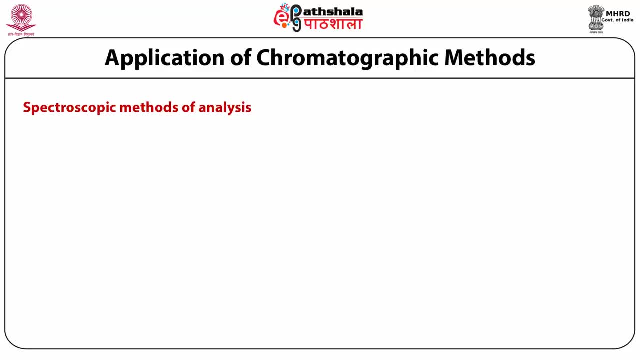 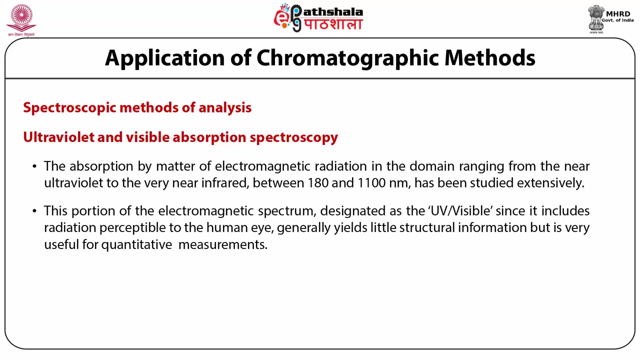 analysis. the number one spectroscopic method is ultraviolet visible absorption spectroscopy. the absorption by matter of electromagnetic radiation in the domain ranging from the near ultraviolet to the very near infrared, between 180 to 1100 nanometer, has been studied extensively. this portion of the electromagnetic spectrum, designated as the 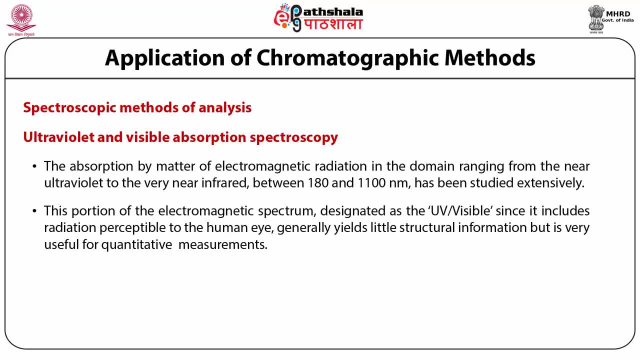 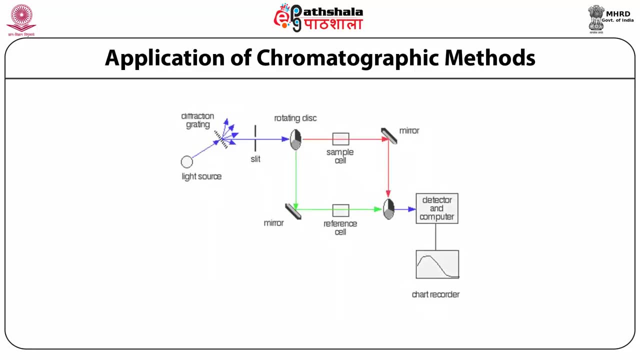 UV visible, since it includes radiation perceptible to the human eye, generally yields little structural information but is very useful for quantitative measurement. here is the schematic representation of UV visible spectrophotometric technique in which the deuterated lamp or the tungsten lamp is used as a light source of UV visible range. then this light is passes through the diffraction. 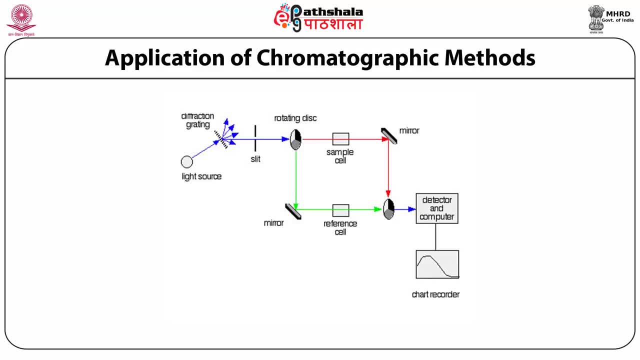 grating or the monochromator, which absorbs the other irradiated light and only absorbs the light, which absorbs the other irradiated light and only absorbs the other irradiated light and only absorbs the other irradiated light and only desired wavelength- is passing through the reference cell or the sample cell, then this beam of light 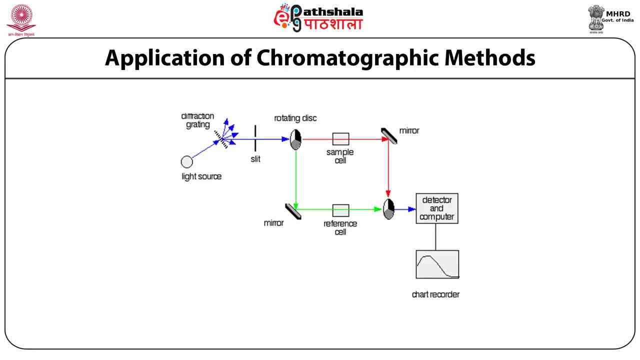 is splitted and one beam is passing through the reference cell that contain the blank or the distilled water to subtract the impurities present in the regenerating solvent, and another beam is passed to the sample cell which contain the absorbing sample so that it these sample absorb the UB visible radiation. where the beam and lose light. we profile the赤 beam of light which contains the absorbing sample, so that it these samples absorb the UV visible radiations. the beam is passed to the sun and it contains the incoming water, which contains the sample sample and this black produced based sample so that it these sample absorbs the UV visible radiation. 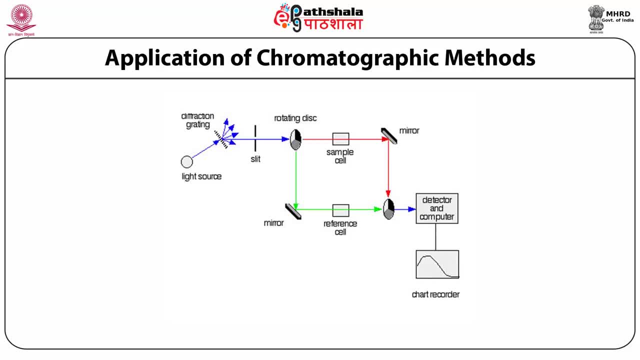 monsieur, greetings. to fall in the target security, you are sitting worried about the panel position which is one time to be maintained I area 24に. are you ready to follow the incident relates: specific procedure. recording this presentation ici. radiations and the transmitted light is detected by the detector is generally. 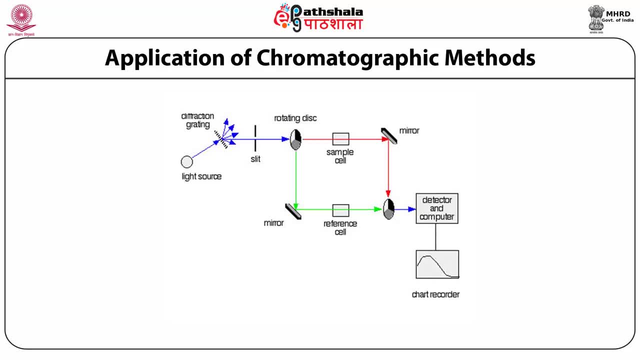 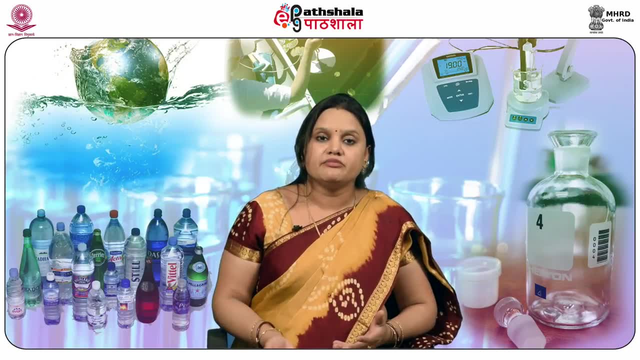 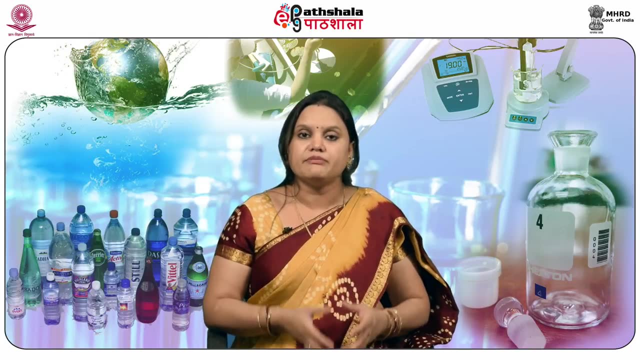 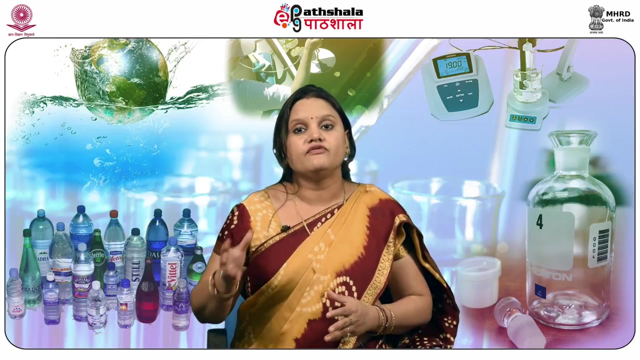 photo tubes or photo multiplier tubes are used here as a detector. the concentration of an analyte in a solution can be determined by measuring the absorbance at some wavelength and applying the Lambert Spears law. the method is known as calorimetry and considered as the workhorse of many. 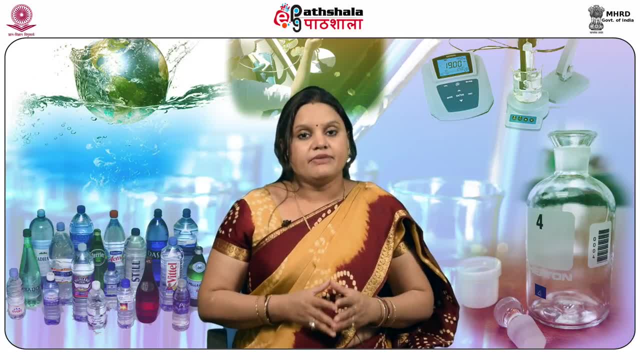 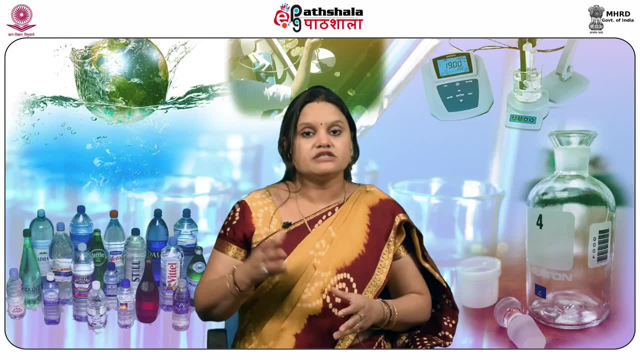 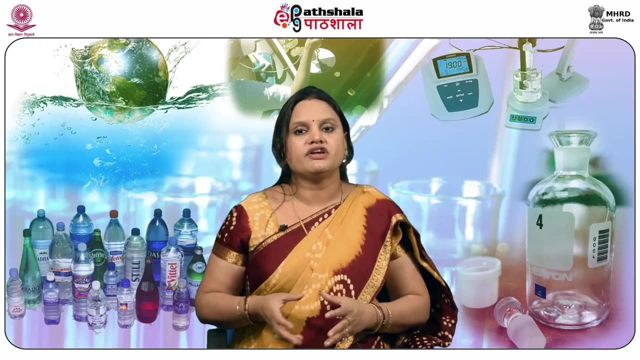 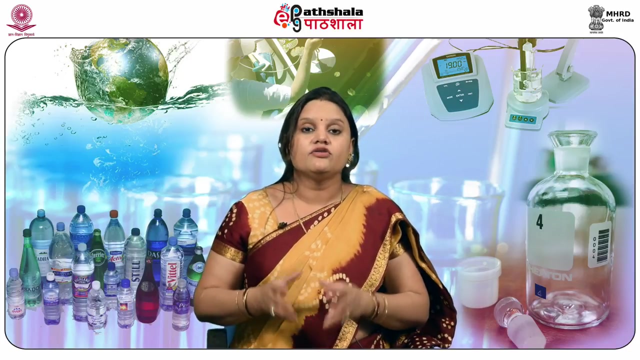 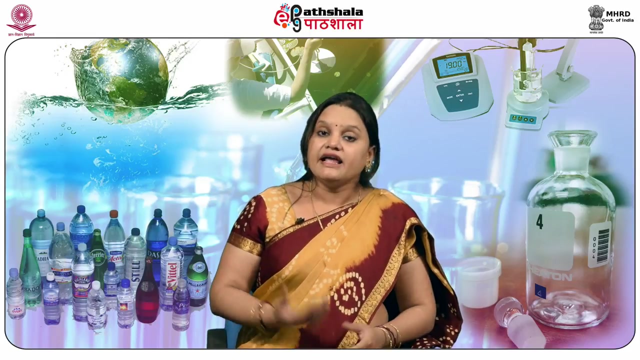 laboratory colorimetry applies not only to the compounds possessing and absorption spectrum in that spectral region, but equally to all those compounds which, following modification by specific reagents, lead to derivation- ah, ah, lead to derivatives- which permits absorption measurements. The next method that we are discussing here is the infrared spectroscopy, The analytical 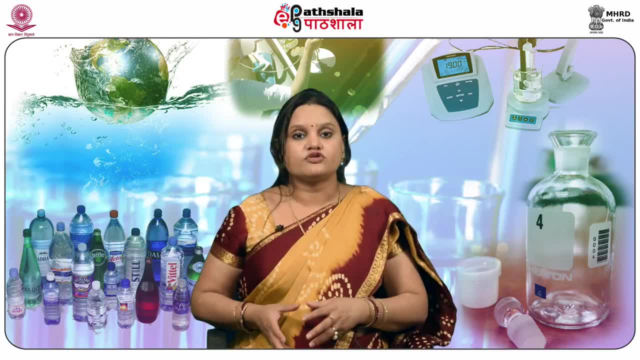 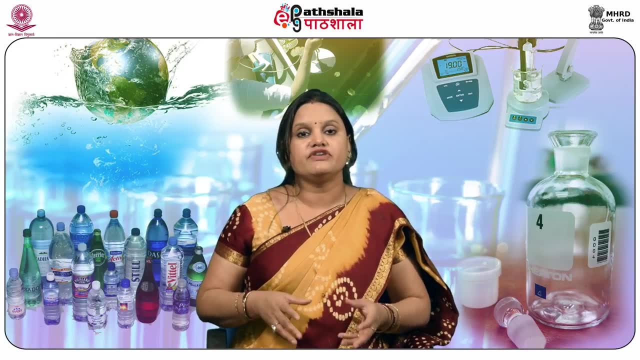 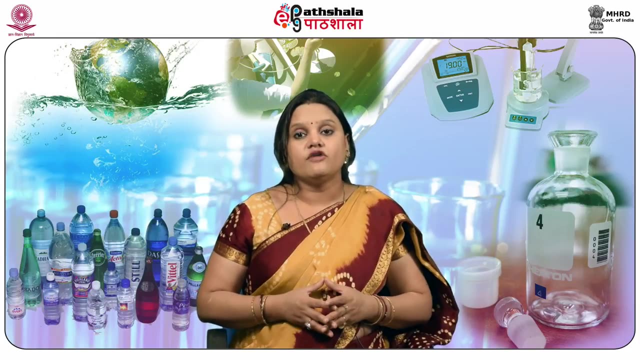 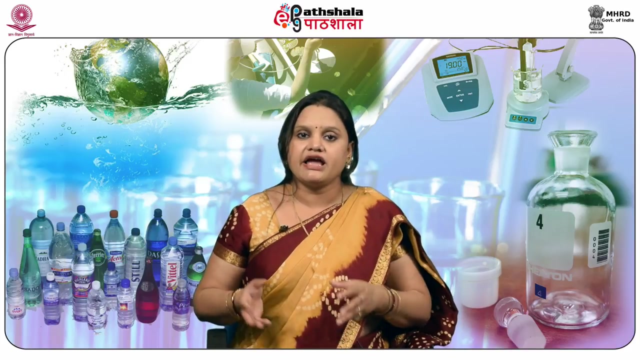 infrared studies are based on the absorption or the reflection of the electromagnetic radiation that lies between 1 and 100 meter. 1 to 1000 meter. This is one of the most common spectroscopic technique used for compound identification and measuring of the concentrations in many samples. 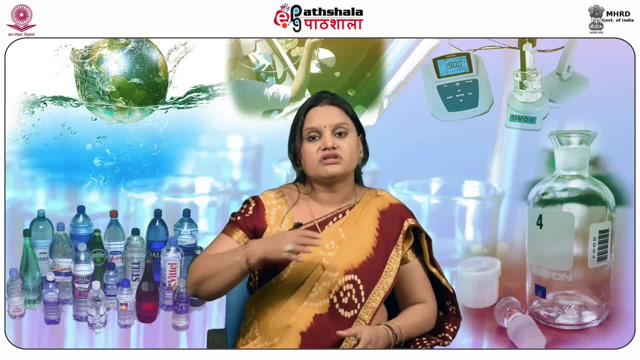 This spectral range is subdivided into three smaller area: the near infrared region, that lies between the 1 to 20 meter range. and the near infrared region that lies between the 1 to 20 meter range. and the near infrared region that lies between the 1 to 20 meter range. and the near infrared. 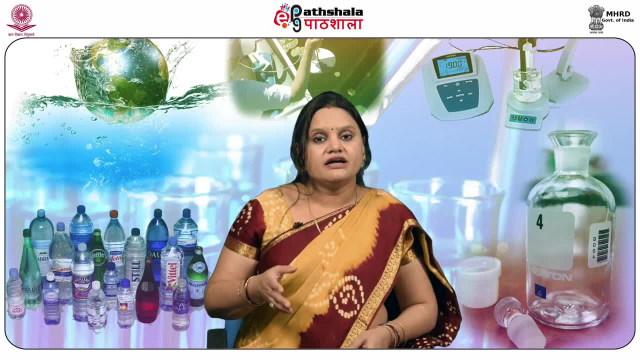 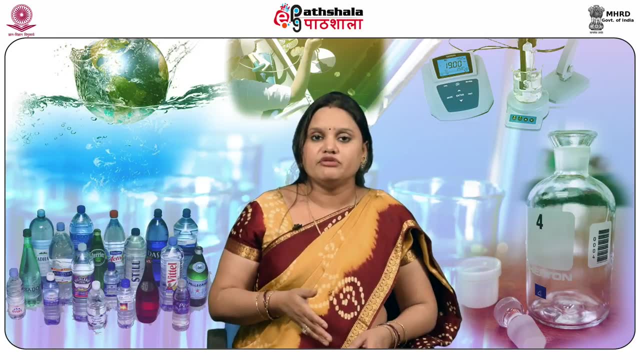 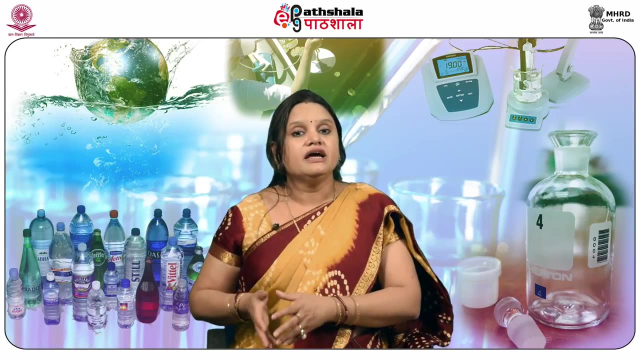 region that lies between the 25 to 50 meter range center, the mid infrared region that lies between the 20 to 50 meter range center and the far infrared region that is beyond the 25 meter. Although the near IR is poor in specific absorption, it is considered as an. important method by quality control laboratories for quantitative applications. By contrast, the mid IR region provide more information upon the structures of the compounds and consequently it is much used as a produce. it is much used as a procedure for identifying organic compounds, for which it remains a form of functional group finger printing. 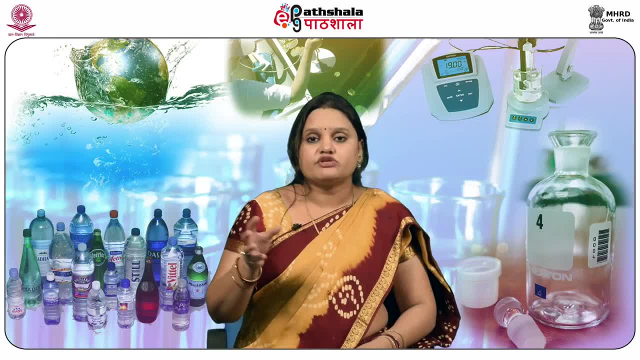 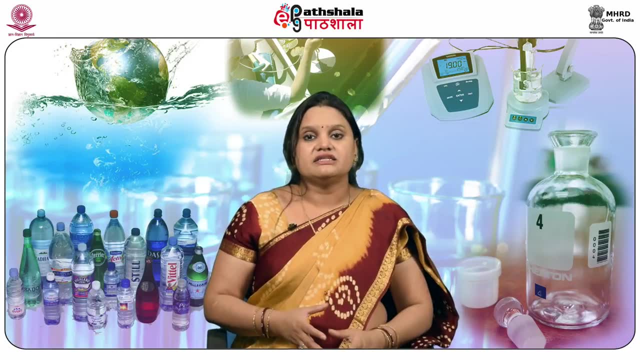 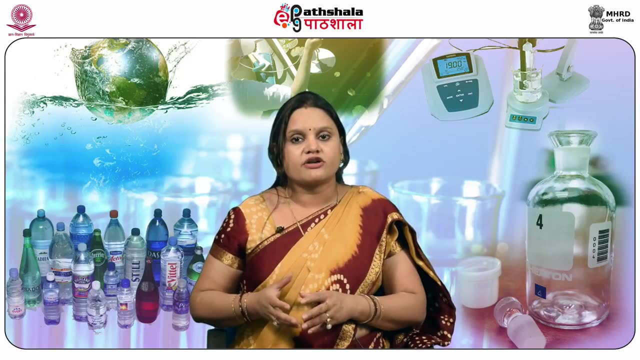 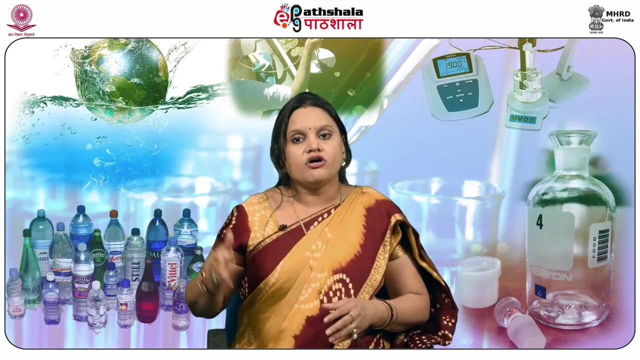 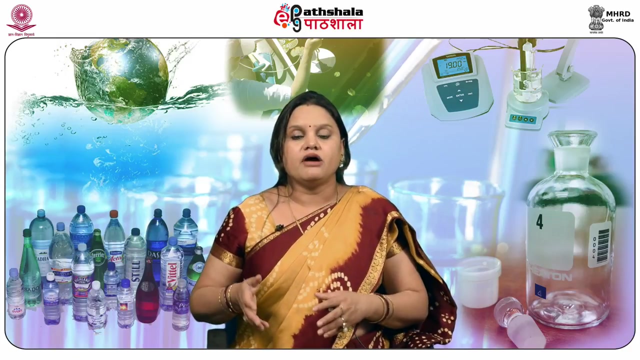 The far IR requires the use of specialized optical material and sources to conduct these analysis. there is a full range of instruments, from Fourier transform spectrophotometer to a multiplicity of the analyzer of dispersive or non-dispersive type, specialized in the measurement of predefined compound, for example analysis of gases and vapors, or which allow the continuous 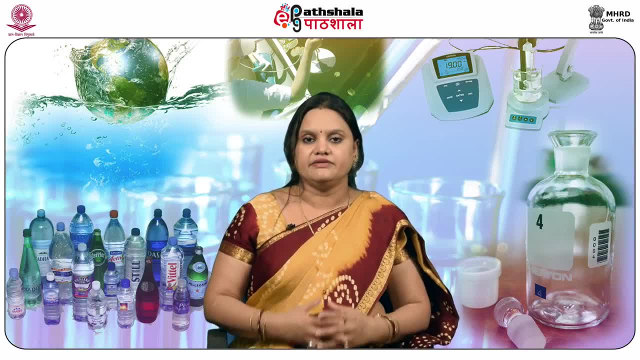 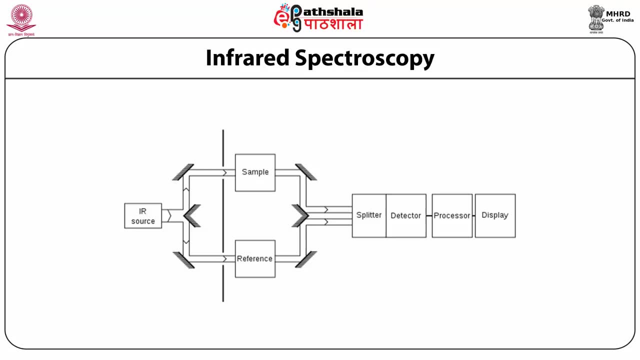 analysis on a production line. this is the schematic representation of IR spectrophotometer where the IR source are used to generate the IR radiation that is passed through the reference and the sample cell simultaneously so that reagent solvent correction can be made by this process. then the sample cell is absorbed the IR radiation which can be 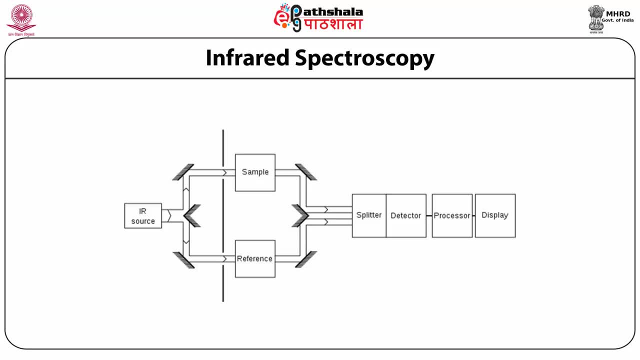 to the detector. there is the photo tubes of photo multiplier tubes are used as a IR source, so the sample- either it will be a solid or liquid- can absorb this IR radiation and the percentage transmittance is determined by this photo multiplier tube detector. the next one is the fluorimetry and the chemiluminescence, the some organic and the inorganic compounds. 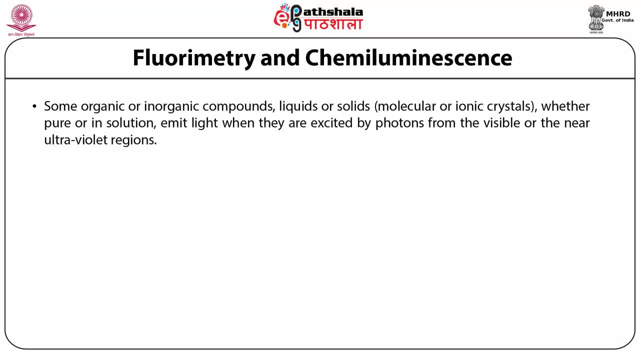 like liquid or solids, like molecular or ionic crystals, whether pure or in solution, emit light when they are excited by photons from the visible or the near ultraviolet regions. among the analytical applications of this phenomena, known as photoluminescence- and this is the principle of fluorimetry, this is a selective and highly selective method of photoluminescence. 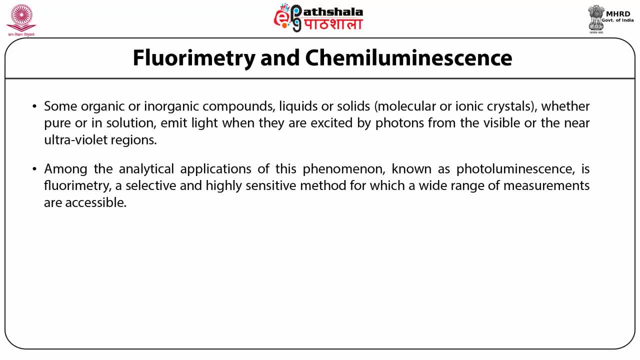 по gorilla-sensor method, for which a wide range of measurements are accessible. the intensity of the fluorescence is proportional to the concentration of the analyte, and the measurements are made with the aide of fluorimeters or the spectrofluorometers. the extremely rapid extinction of the light intensity when excitation seizes is the object of analytes. 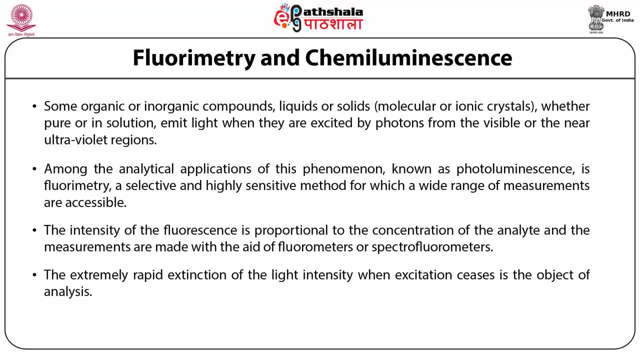 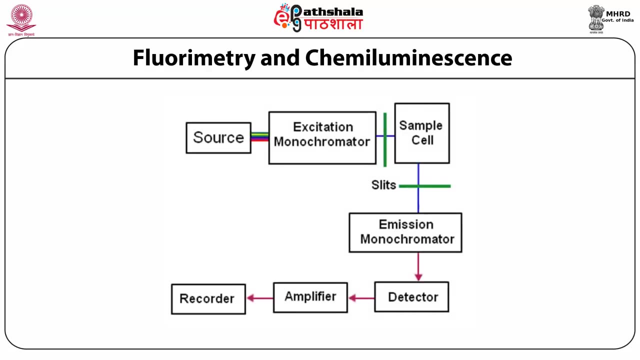 of analysis. by contrast, fluorescence is characterized by a more gradual diminution during time. the fluorescence is equally employed as the basis of detectors used in liquid chromatography. this is the schematic representation of the working of fluorimetry. here the source of fluorescent light is transferred to the monochromator, so that only desired wavelength is passed through the. 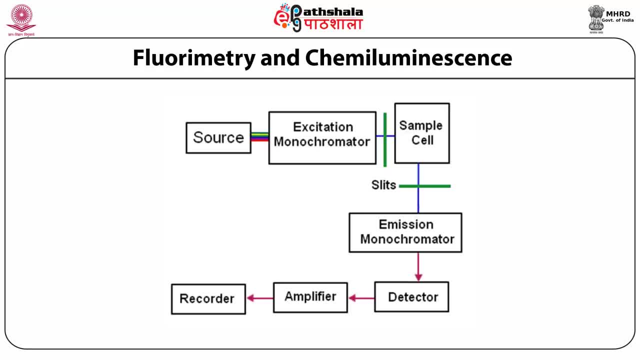 sample cell. in the sample the particles are emitted, the fluorescent light, which is then transferred the emitted light. the second one, monochromator, transfer this emitted light to the detector and then detector identified the concentration of compound by using this emitted light. then amplifier amplifies the signal and recorder record the signal. 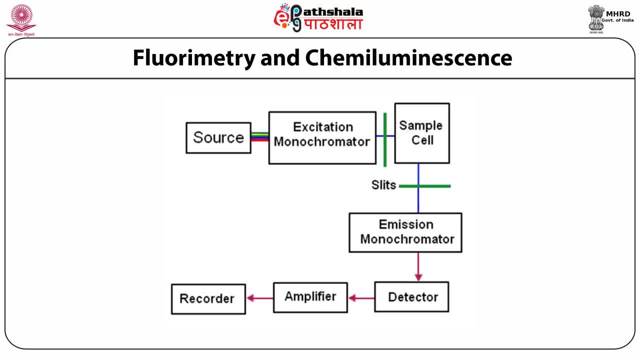 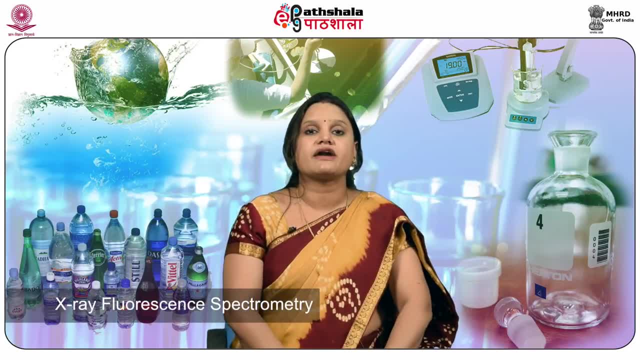 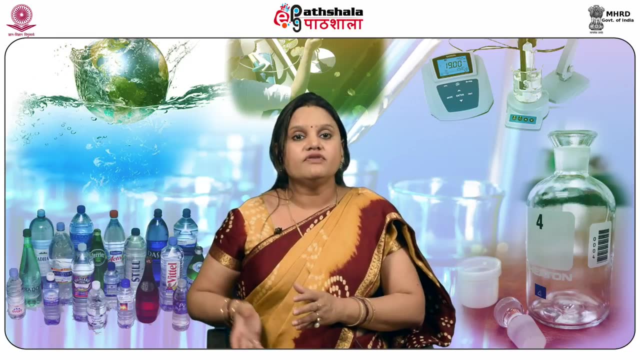 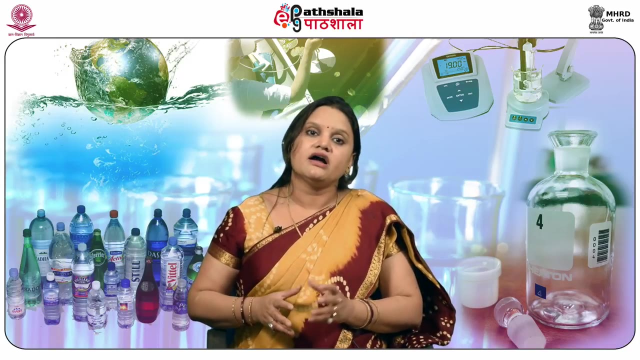 of the impurities present in a fluorimeter. the next method that we are discussing here is the x-ray florescence spectrometry. the x-ray fluorescence is an atomic spectral property universally recognized as a very accurate method, currently exploited under this same name, to provide qualitative and quantitative 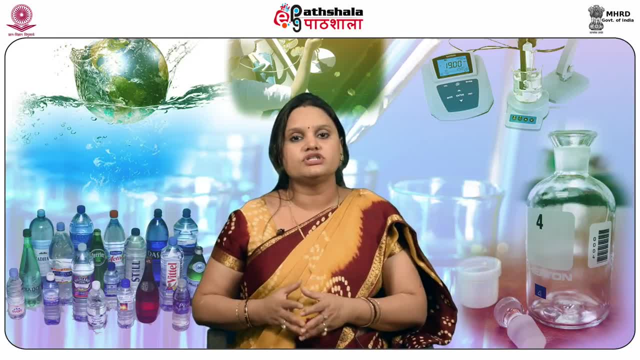 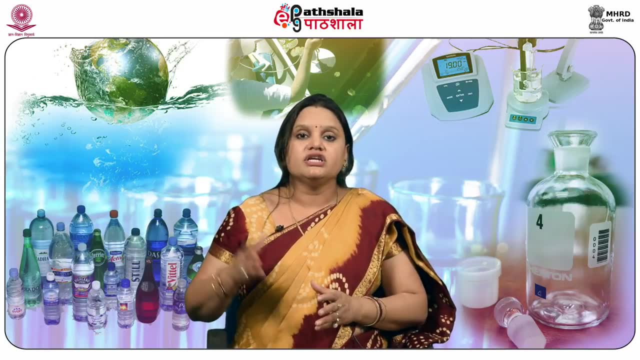 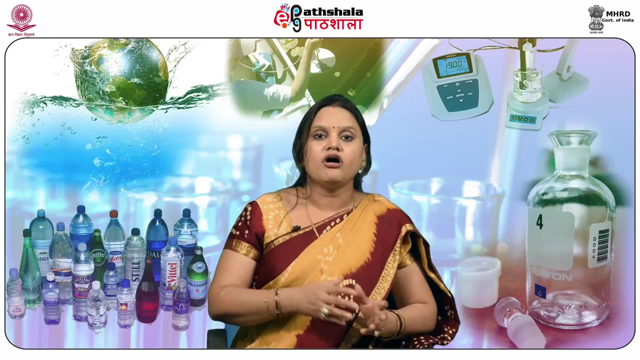 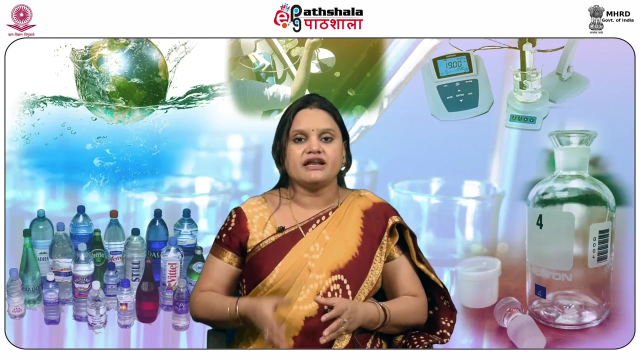 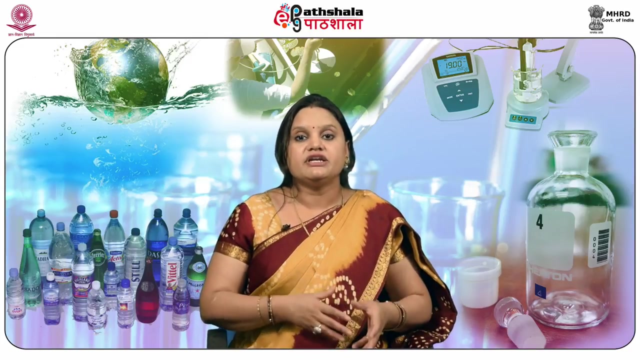 information on the elemental composition of all types of samples. The principle of operation involves irradiating the sample either with an x-ray beam or by the bombardment with the particles, such as electrons, having sufficient energy In order to observe the resulting x-ray fluorescence emitted by the sample. the universal character of this phenomena. 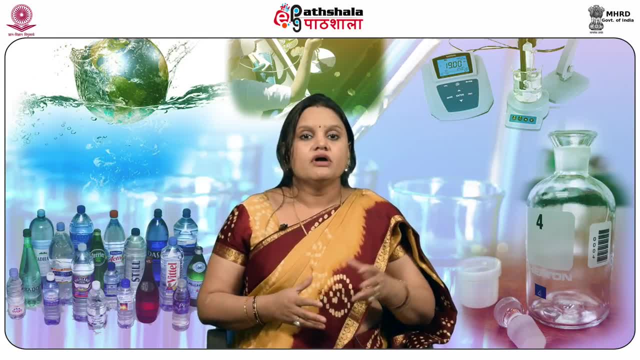 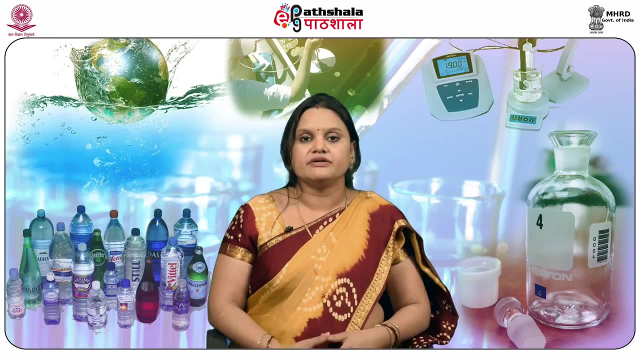 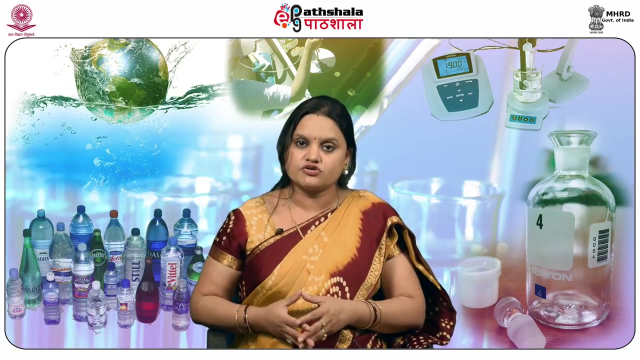 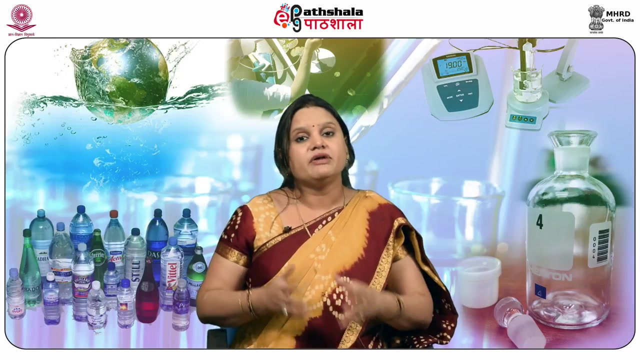 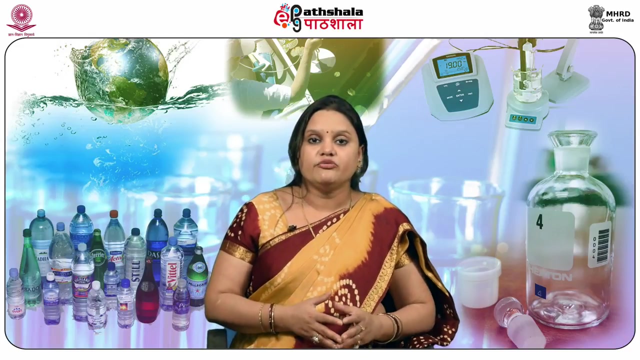 as well as the possibility to rapidly examine samples, most often without preparations, explains largely the axis of this non-destructive analytical method. The technique: The technique encompasses a wide variety of instruments ranging in size from portable analyzers for instant analysis to high-resolution spectrometers, including. 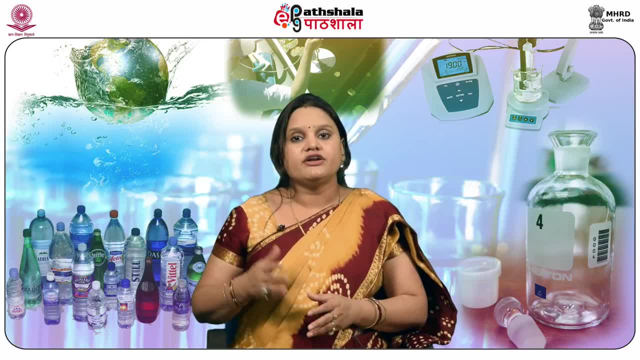 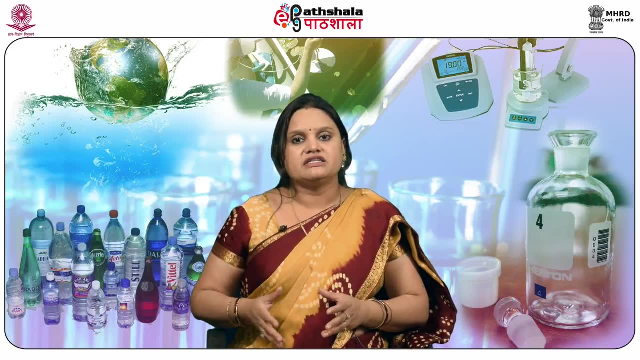 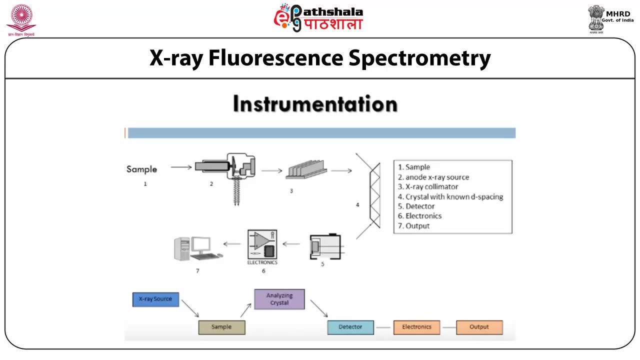 x-ray probes fitted to scanning electron microscopes to make specified analyses or a map. The technique of the elements present here is the schematic representation of x-ray fluorescence spectrometry in this method. the number one here is the sample. the second one is the anode x-ray source. third is the x-ray collimator. fourth is 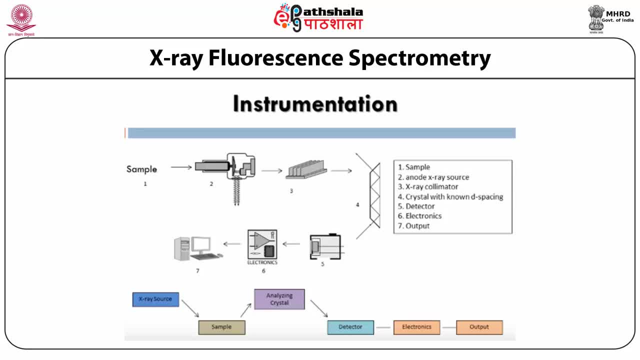 the crystal, known D spacing. fifth is the detector, six is the electronic devices which is used to amplify the signal, and seven, one is the output. so in this instrument, when the x-ray sources passes, the emits the x-ray radiation which is passed through the sample and the radiation which is transmitted from the 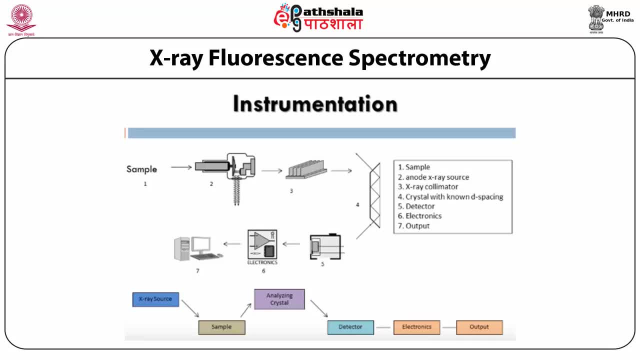 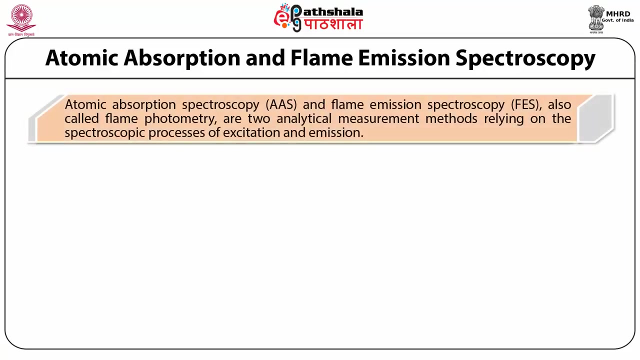 sample cell goes in a analyzing crystal where the different types of bending are done by the D spacing crystal and after that this radiation are detected by the detector and shows as a output signal through the computer. the next is the atomic absorption or the flame emission spectroscopy. the atomic 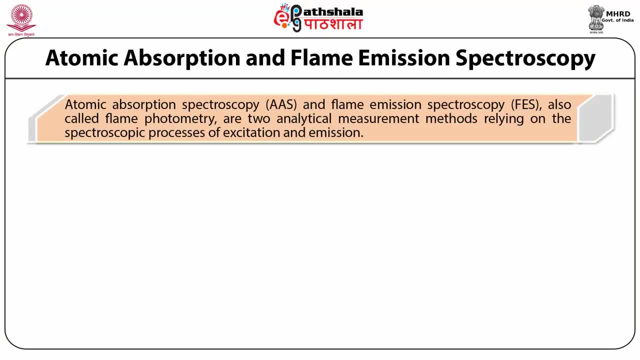 absorption spectroscopy is also known as AS, and the flame emission spectroscopy is known as FES, also called full flame photometry, are the two analytical or the measurement methods relying on the spectroscopic processes of excitation and emission, the methods of quantitative analysis only, and they 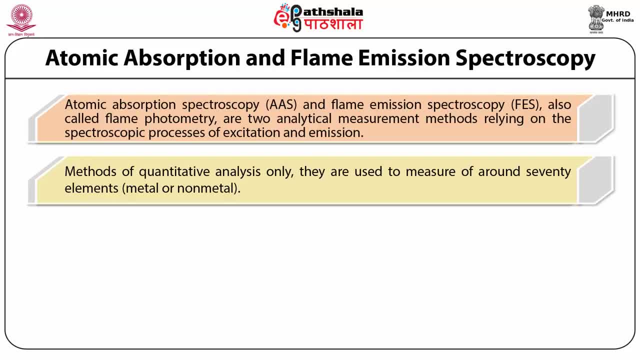 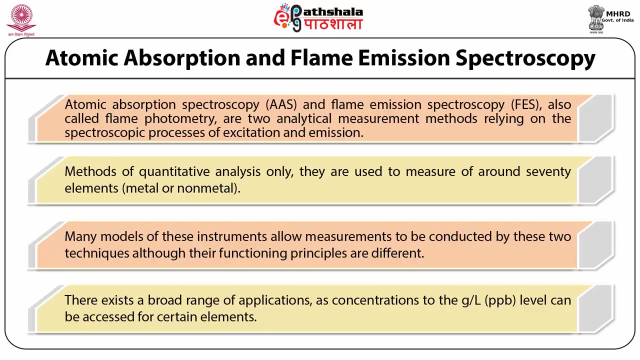 are used to measure the around 70 elements, metals or non-metals. many models of these instruments allow measurements to be conducted by these two techniques, although their functioning principles are different. there exists a broad range of applications, as concentration to the gram per liter, that is, ppb- level, can be assessed for certain elements, generally heavy metals. 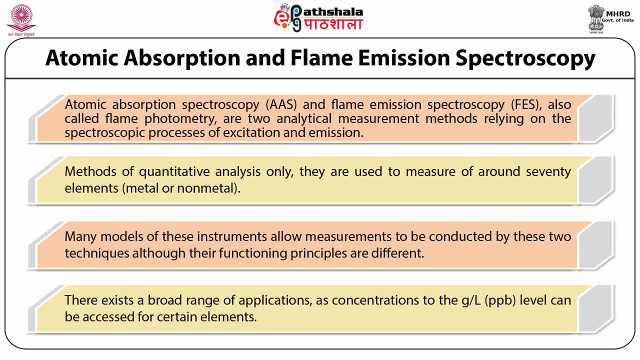 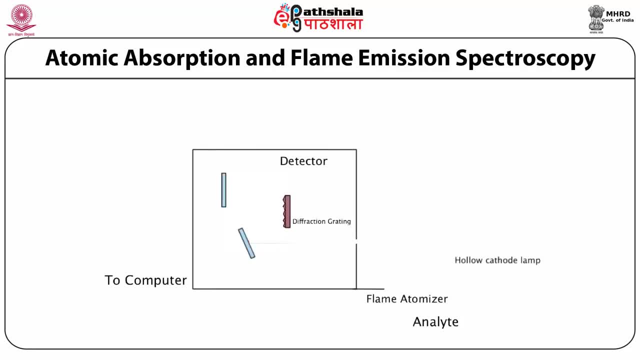 and the rare earth metal can be analyzed by using this absorption technique. this is the picture of atomic flame photometry or atomic absorption spectrophotometer, from where the analyte is entered through the in the flame atomizer and it is burned out at the very high temperature so that the particles of the metal is atomized and goes. 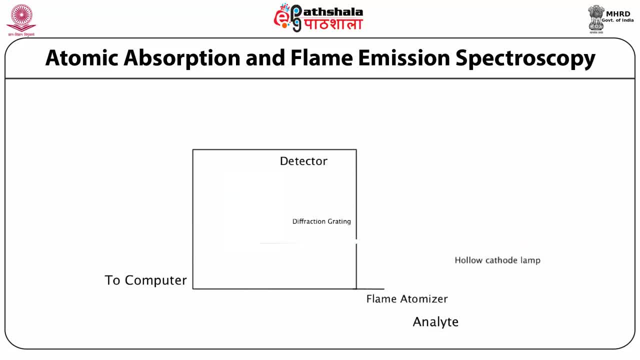 into the higher energy state and when we pass through the beam of light by the hollow cathode lamp at that frequency they are atomized. then they absorb light and goes down to the ground level and this change in the difference in the light and the energy of the light is very important for the 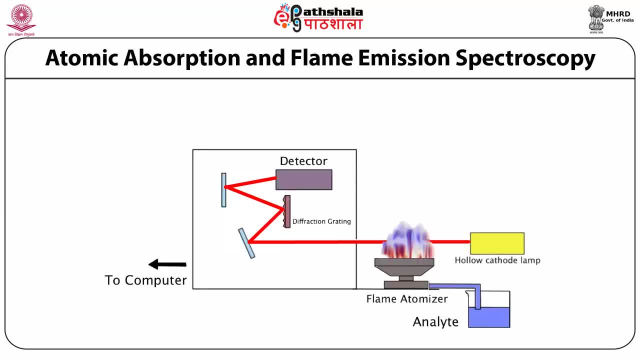 transformation of the metal from the ppb level to the ground level and this change in the difference in the energy level it is detected by the detector and that is again it is converted into the concentration of a substance present in the solution. so most of the trace metals or the other rare earth metal can be determined by 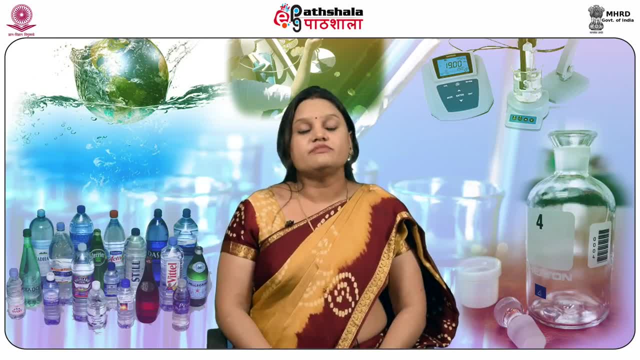 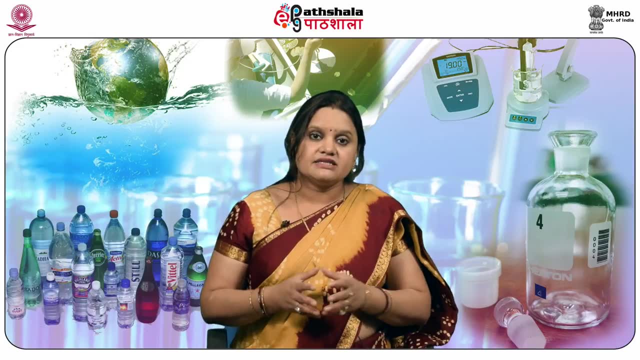 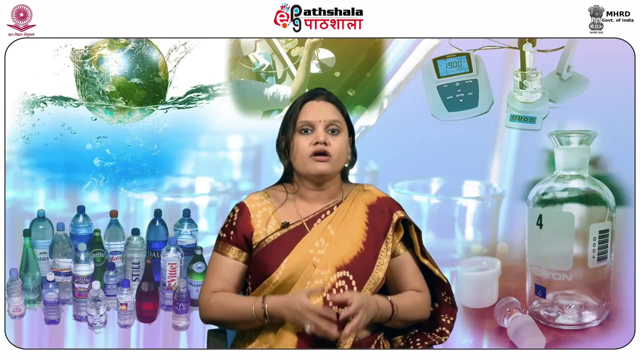 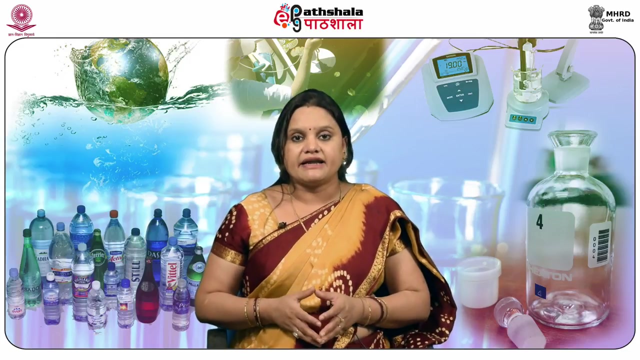 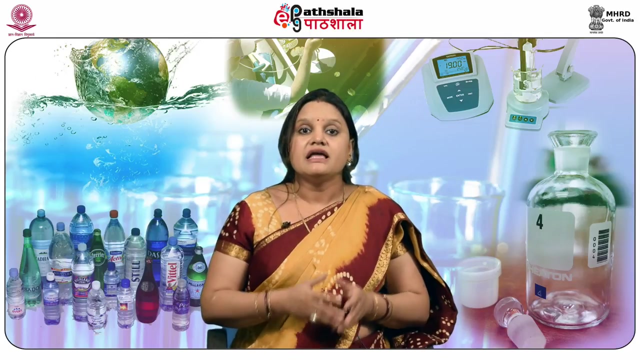 using this technique. the next method that we are discussed here is the atomic emission spectroscopy. the analyzes by atomic emission spectroscopy constitutes a general method for measuring elements on the study of the radiation emitted by their atoms present in an excited state, usually following the organisation. several procedures are used to break down the 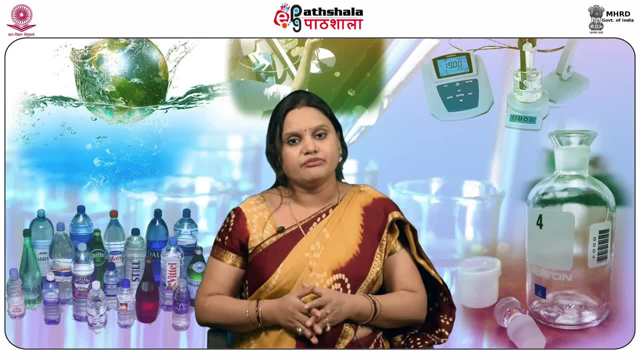 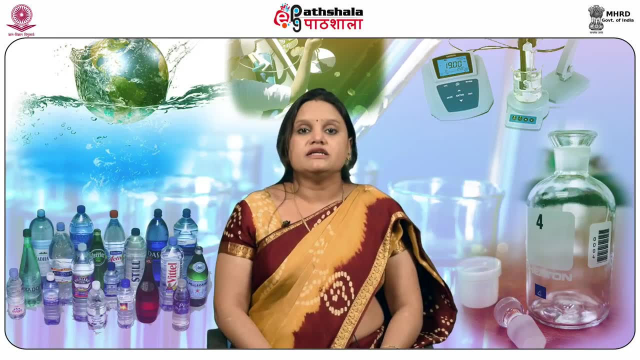 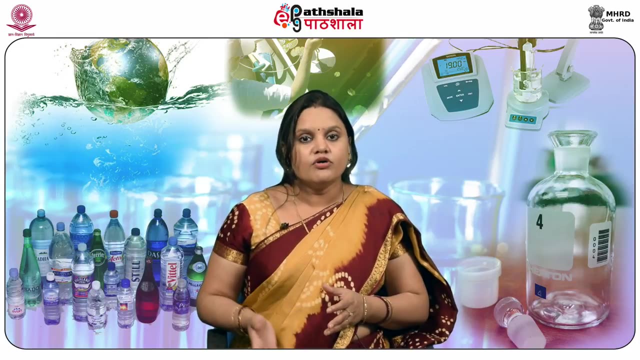 samples, tomatoes and offsets to decomp costume and add planeta Як in their to their constitutive elements, most notably by the effect of high-temperature plasmas, spark sources or glow discharges, the emission being far more complex than those of flame. 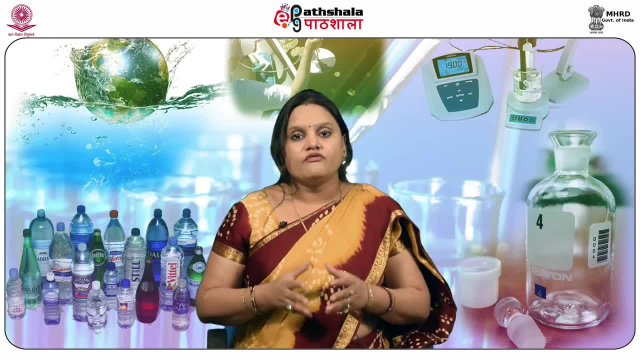 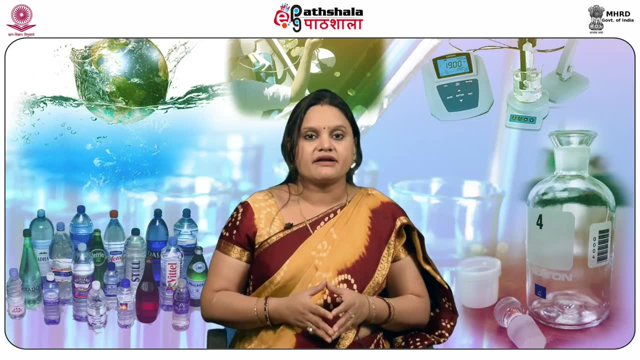 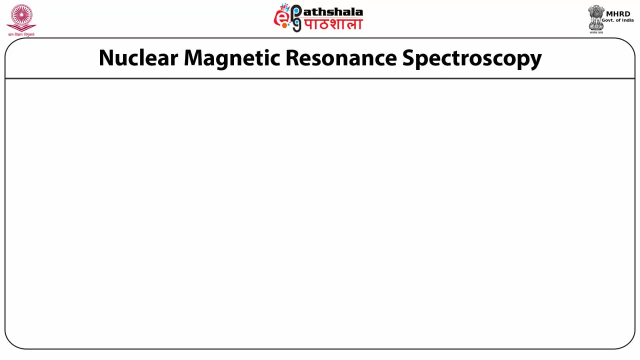 emission and the instruments required- very high-quality optics- to resolve interferences from both spectral lines and the matrix effects. Next one technique is the Nuclear Magnetic Resonance Spectroscopy. The NMR is a powerful and theoretically complex analytical tool that allows the study of compounds. 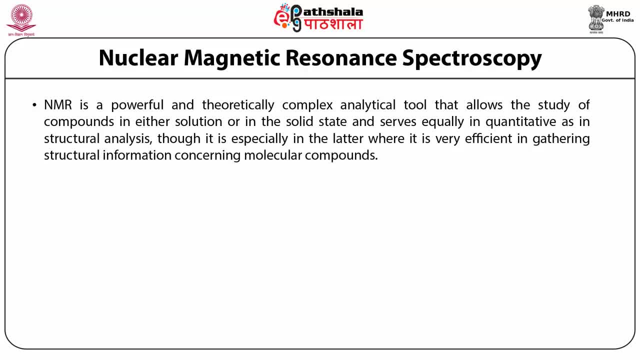 in either solution or in the solid state, and serves equally in quantitative as in structural analysis. Though NMR is a complex analytical tool, NMR can be used in many ways. It is especially in the latter where it is very efficient in gathering structural information. 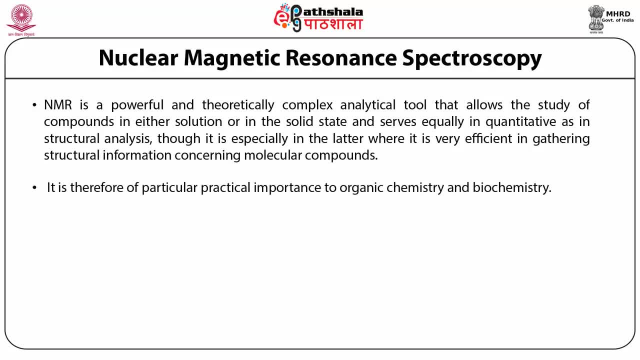 concerning molecular compounds. It is therefore of particular practical importance to organic chemistry and biochemistry and used as a complementary technique to methods of optical spectroscopy and mass spectrometry. It leads to precise information concerning the structural formula and the stereochemistry, and, in some cases, the preferred conformation of molecules, and even to the identity of the. 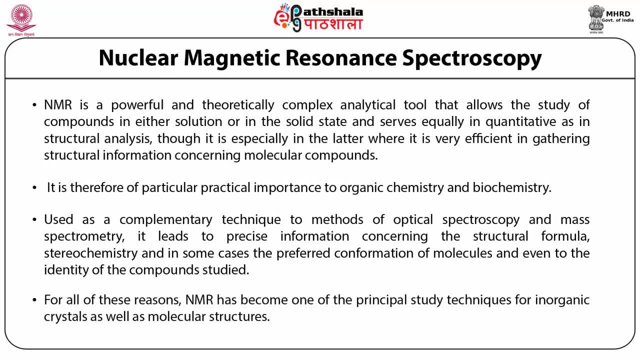 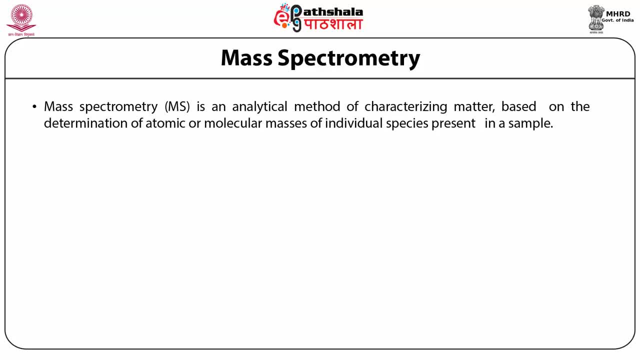 NMR can be used in many ways. NMR can be used in many ways. NMR can be used in many ways of atomic or the molecular masses of individual species present in a sample. The instruments employed for carrying out mass spectrometry can be classified into different categories. 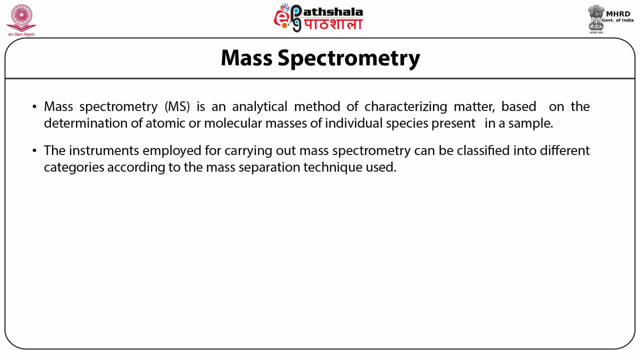 according to the mass separation technique used. The sum are derived from assemblies developed at the beginning of the 20th century for the study of particles or ionized atoms submitted to a magnetic field, while others rely upon different principles. The continuous improvement have made mass spectrometry the most versatile and widely used analytical method available today. 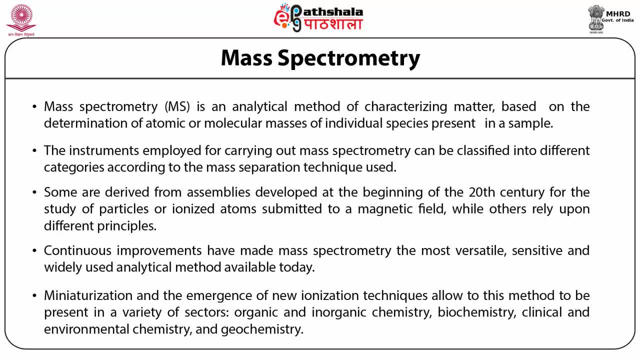 The miniaturization and the emergence of new ionization techniques allow to this method to be present in a variety of sectors like organic and inorganic chemistry, biochemistry, clinical and environmental chemistry and geochemistry. Now this technique is also equipped with the other techniques like gas chromatography or the high-performance liquid. 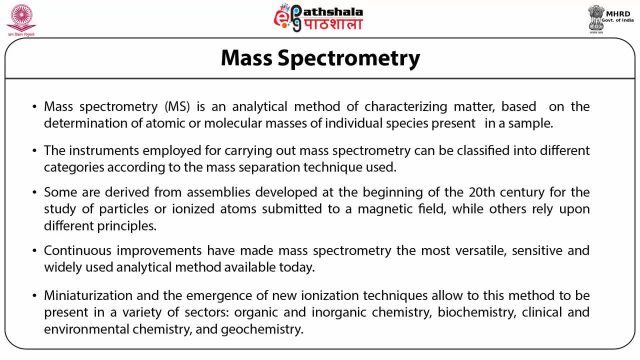 chromatography, so the their sensitivity of those instruments increases by connecting with the mass spectrometer. The mass spectrometer is also used in the mass spectrometer. The mass spectrometer is also used in the mass spectrometer. The mass spectrometer is also used in the mass spectrometer. 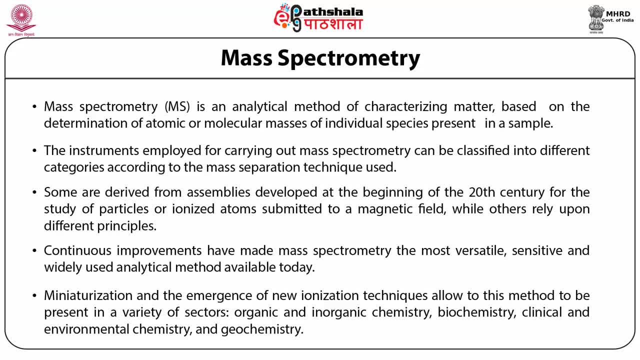 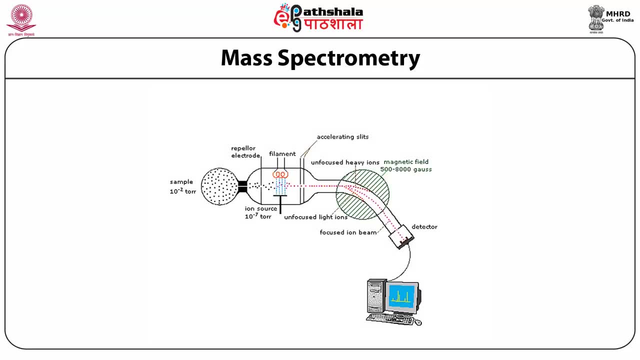 and these combination of these two techniques are frequently used to analyze various types of environmental contaminants in the soil and the water sample. Here is the schematic representation of mass spectrometry where the sample is passed through the vacuum chamber where the ionization of sample takes place and the fragments- ions- are passed through the 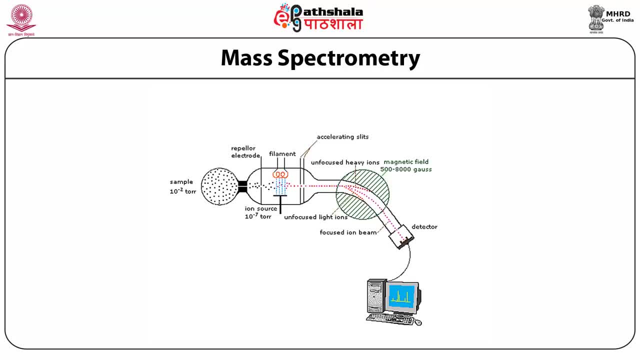 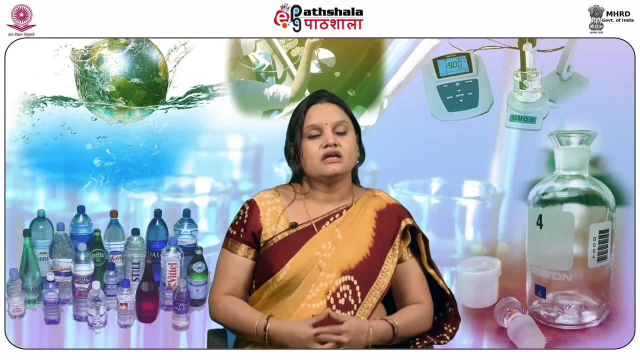 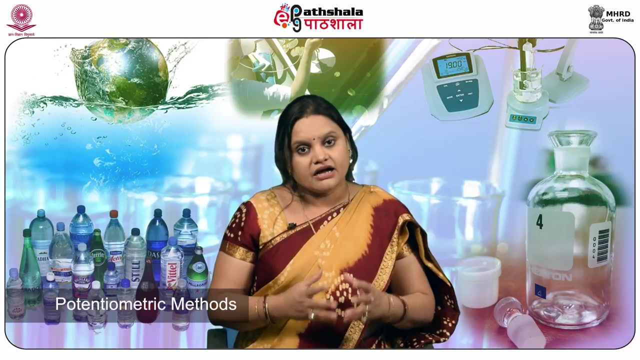 the quadrupole system, from where the unused ions are settled out and only desired ion are, passes through the detector, which is detected substance present in the sample, and then it is displayed by using the computer. Now we discuss here the next procedure, that is, potentiometric method. a great deal of quantitative measurements in chemical analysis are based on electrochemistry, called electrochemical methods. They can be separated into two categories: those based upon the measurement of potential, that is potentiometry, and those which are exploit the measurement of current, that is voltammetry. The first group, which is developed in this chapter, use the ion selective method. 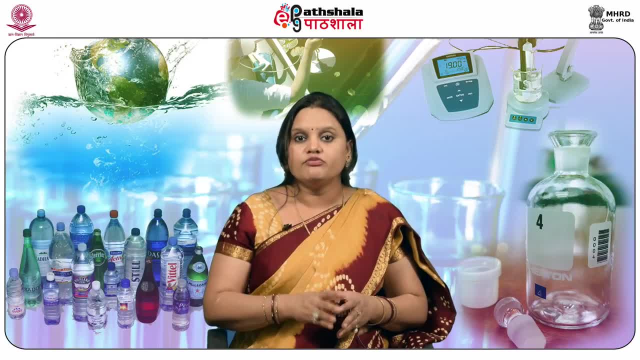 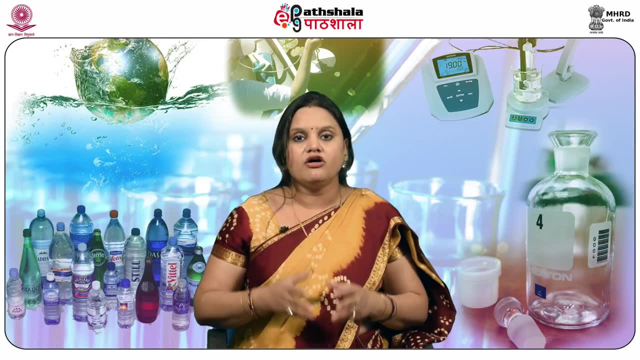 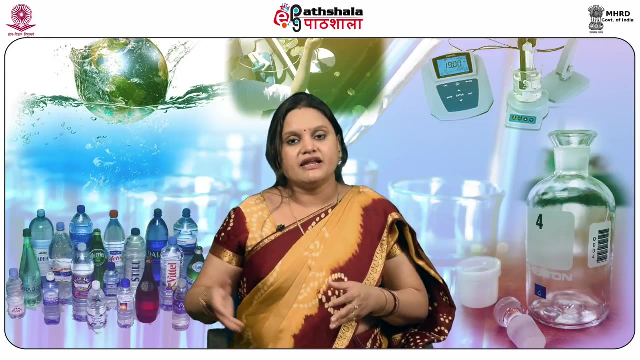 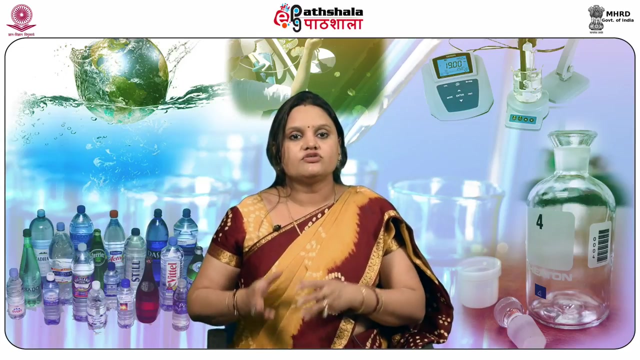 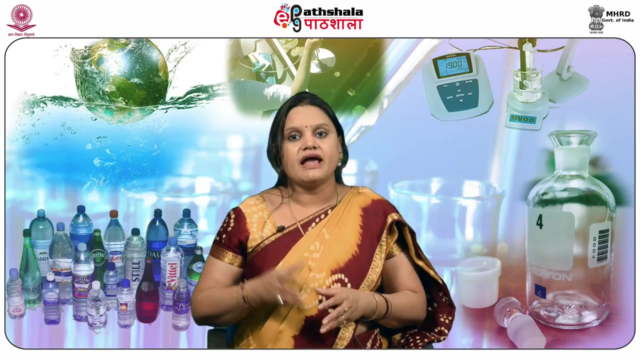 The first group which is developed here used ion selective electrode, and the principle of these chemical sensors is to create an electric cell in which the analyte behaves in such a way that the potential difference obtained relates to its concentration. The measurement of pH, the most common and the best known electroanalytical method, is part of this group. 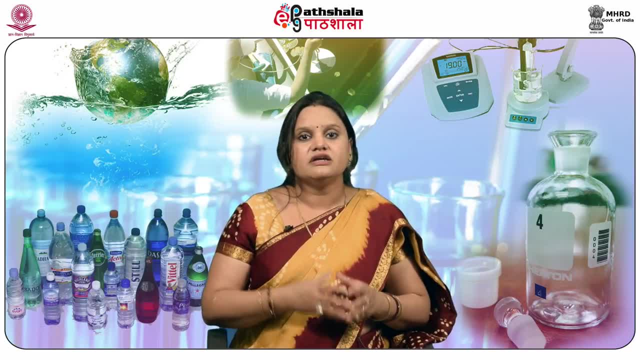 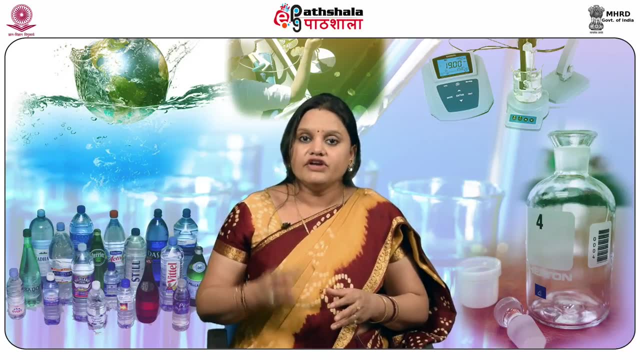 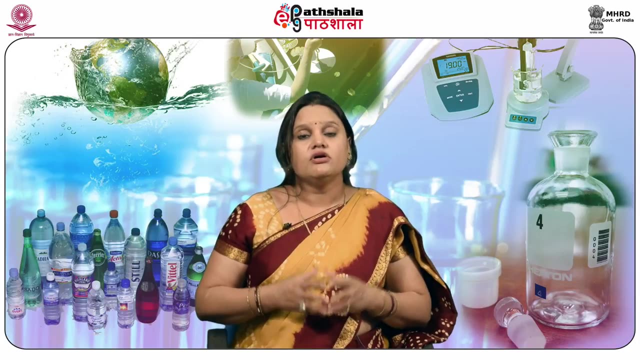 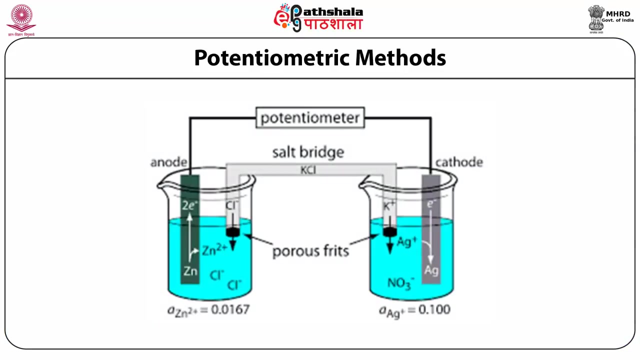 The most of the measurement concern the determination of ion in aqueous solution through the particular electrodes with selective membrane also allow the determination of molecules. So these potentiometric method nowadays are using as a selective method for the analysis of various type of water pollutant sample. This is the picture of 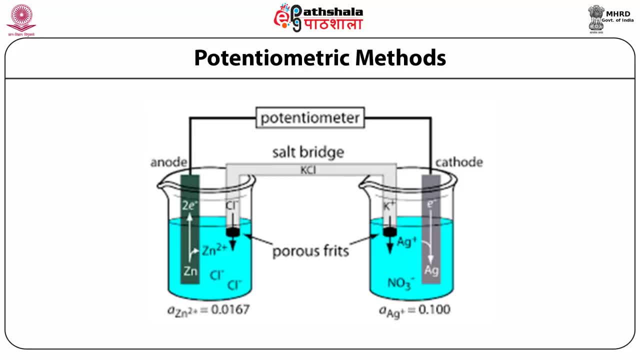 potentiometer where the two electrodes are dipped in a different solution and they are working as anode and cathode, and here in between the salt bridge is used. These types of electrodes are used for the analysis of various types of water pollutant, and these types of potentiometer are also used as a fuel cell for the generating energy in the. 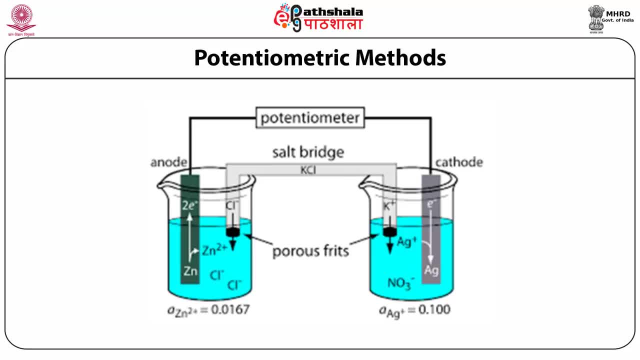 remote areas and also the potentiometer is also used to purify the water and the other contaminant solution from the ions. When we passes the current, then the both the electrode ionize the electrolyte solution and the electrodes are passing through the salt bridge and they can. 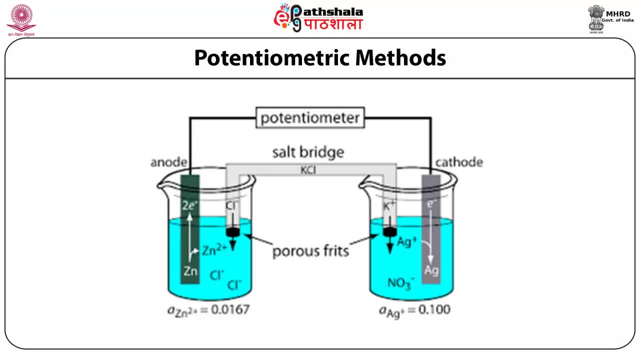 be separated from each other and they can be separated from each other. So this is the solution which is separated and deposited at the surface of the electrode and the remaining solution is going to be clean or the energy also generated by this system, because the electrons are 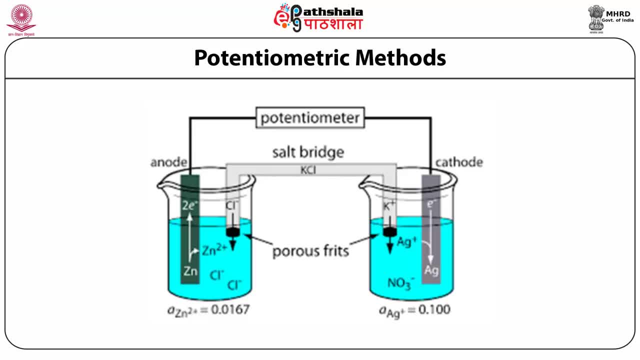 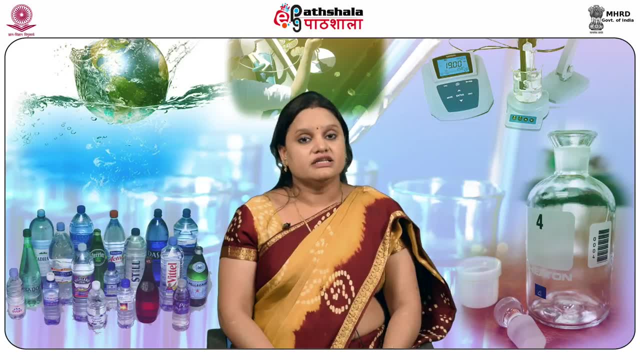 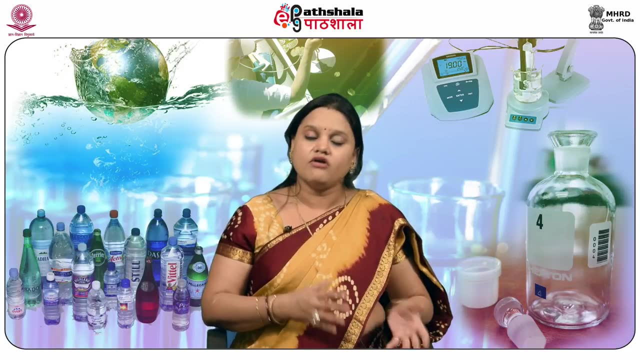 produced here which can be converted into the electric energy. So at the end of this module we discuss here about the detail, discuss here in detail about the different branches of the electrode. The chromatography method is often referred to as the P-physical chromatography of the electrode. 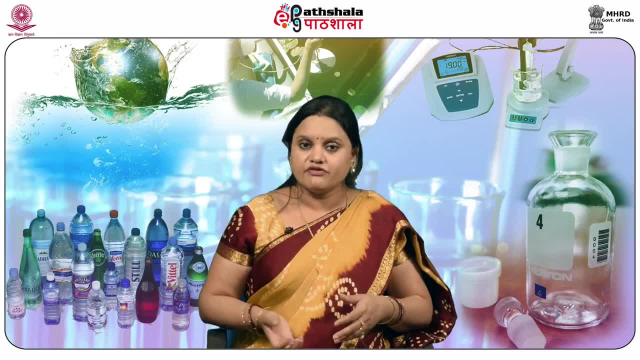 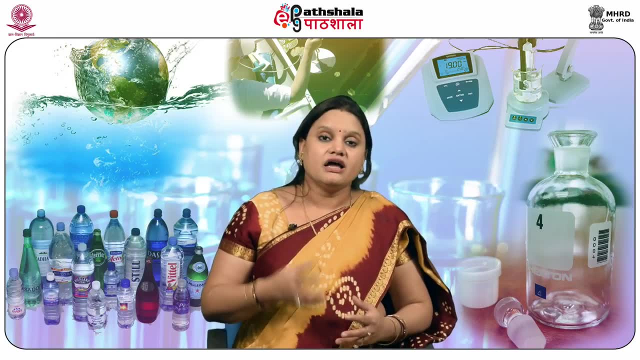 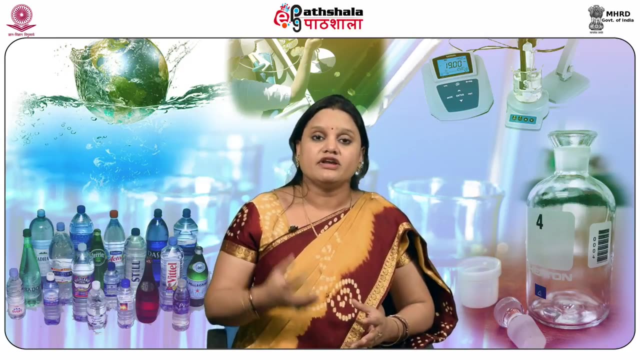 In the past, chromatography method has had many significant branches of analytical chemistry. The chromatographic methods like gas chromatography, thylia chromatography, high performance liquid chromatography, ion exchange and many more methods nowadays used for the analysis of various environmental pollutants and other various types of environmental factors like soil, water, air. 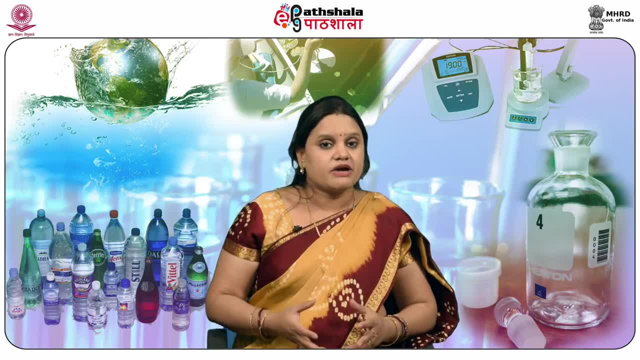 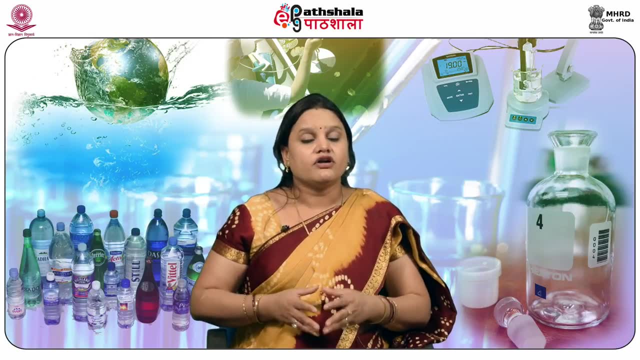 We have also discussed here in detail about the analysis of the initial environmental pollutants- chemo methods can be utilized- as well as chemical quantities of chemical components, as well as in the detail about the various spectroscopic method like IR, UV, AS, NMR for, and their application. 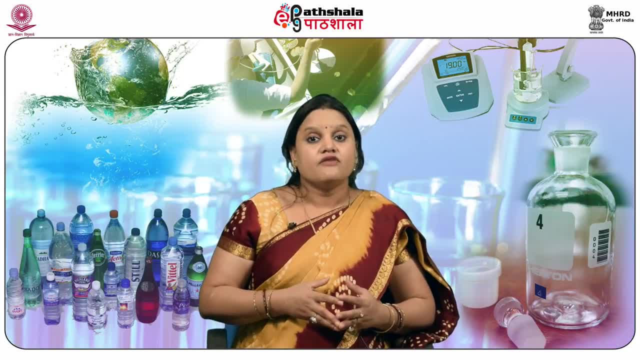 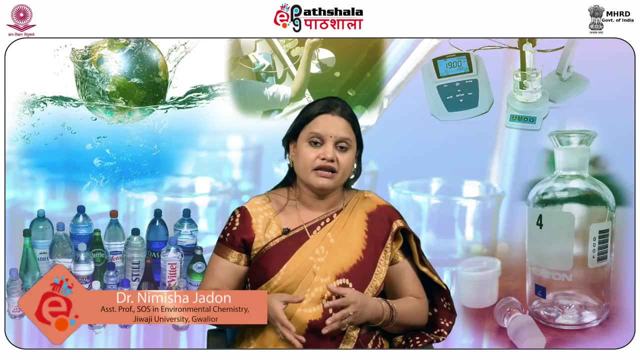 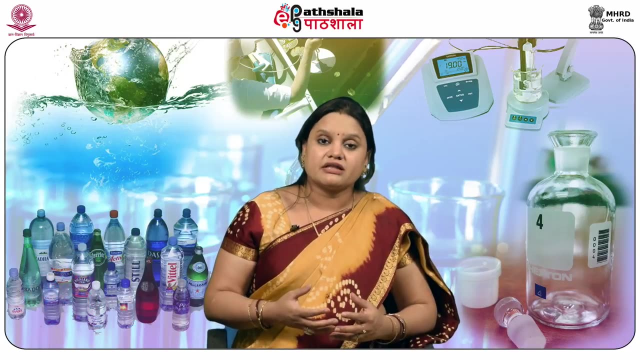 in the analysis of environmental contaminants. We have also discussed here about the application of these methods for the environmental analysis, as well as we have discussed some other electrochemical or the potentiometric method for the analysis of environmental samples. Thank you so much.